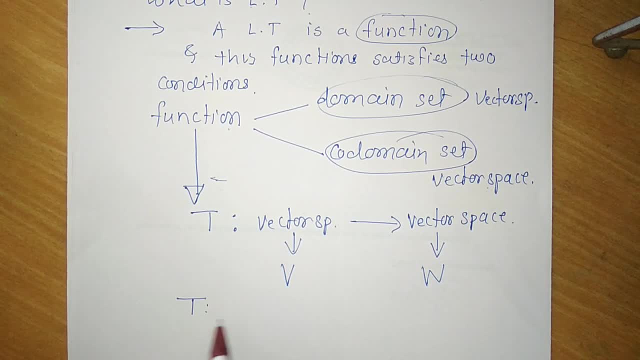 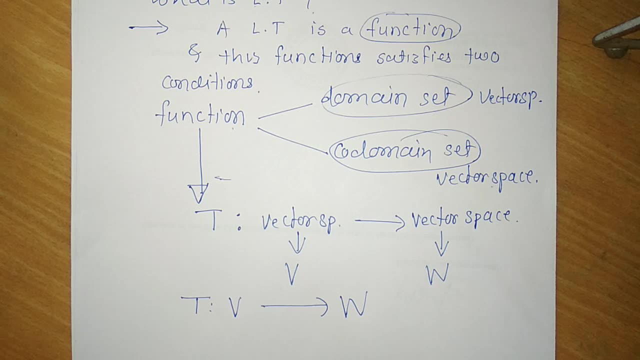 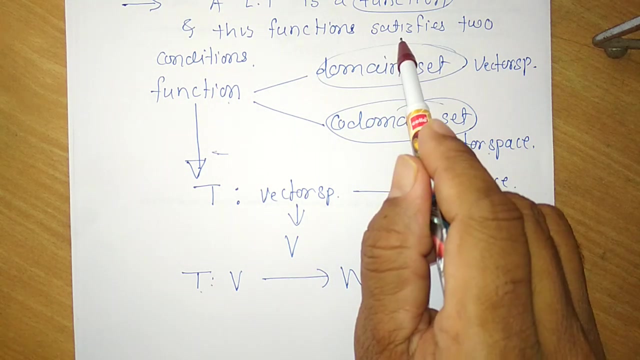 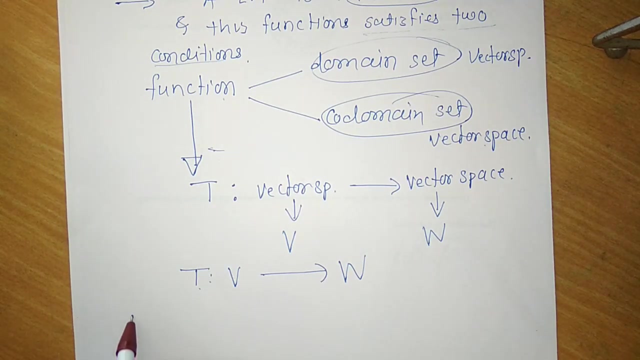 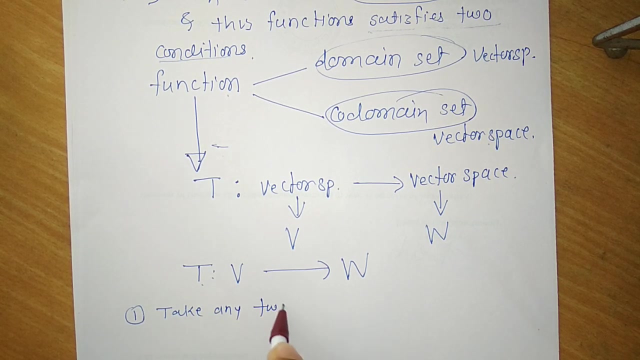 it is denoted by w. So a linear transformation t is a function from one vector space v to w. The next question is: if it is a function, then this function must satisfy the two condition. okay, What are the two condition? The first condition is that take any two vectors in domain set. domain set: okay, that is for. 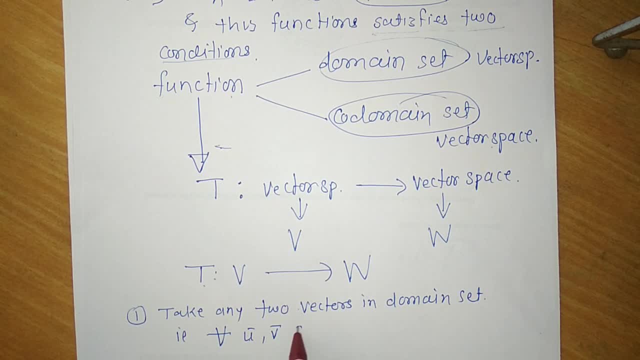 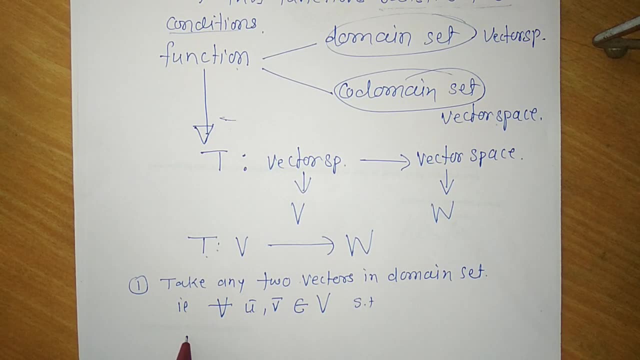 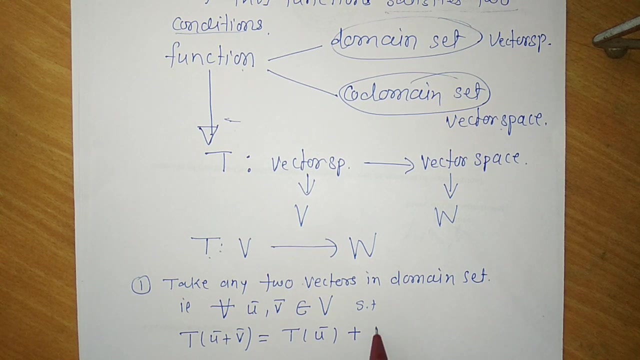 all u bar and v bar. these are the two vectors. any two vector in the v set and such that the condition is t is a function from one vector space to another vector space, v to w. So t of u bar plus v bar is equal to t of u bar plus t of v bar. this is the first condition. 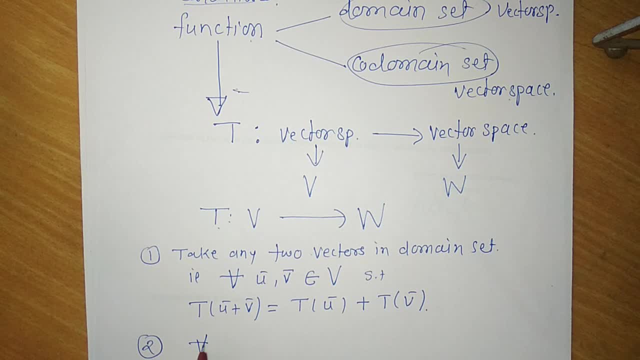 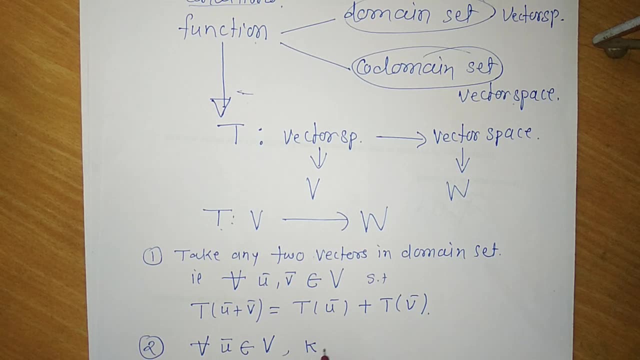 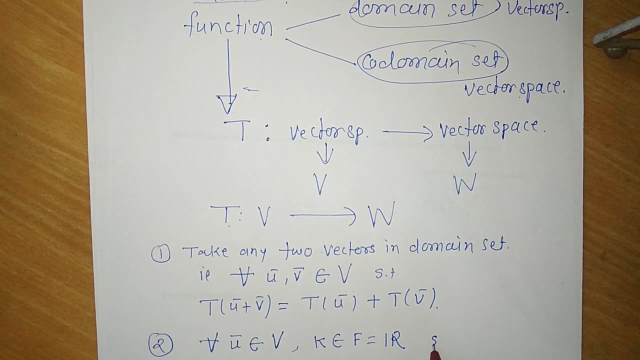 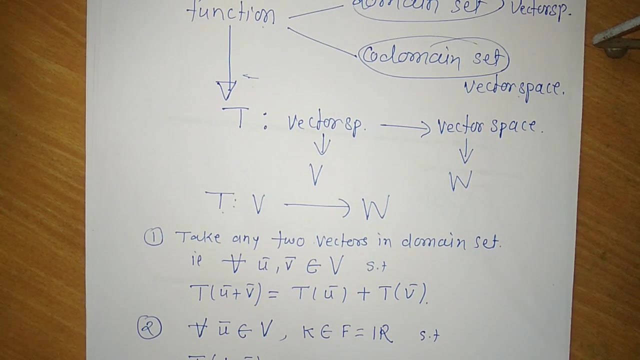 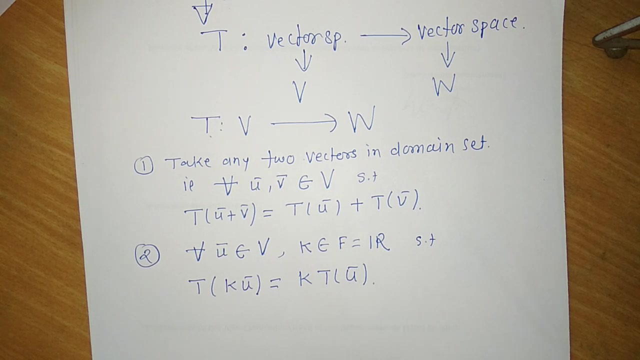 Second condition is that take any vector for all u bar belongs to v, that is the domain set. one of the scalar k belongs to f. So here we take. the field is a real number, r, Such that t of k times u bar is equal to k times t of u bar. 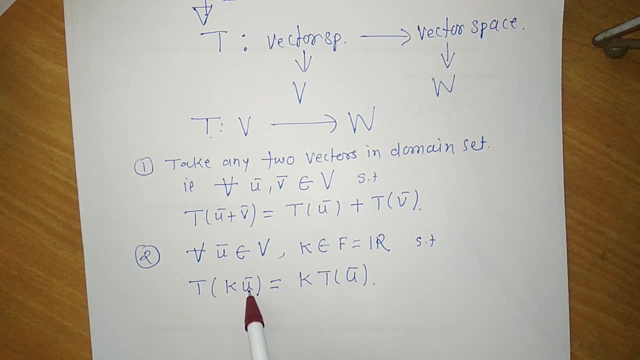 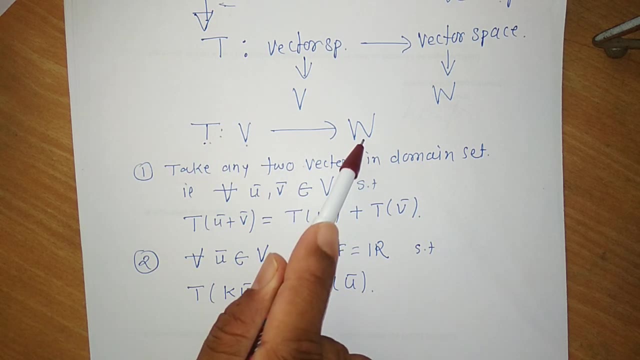 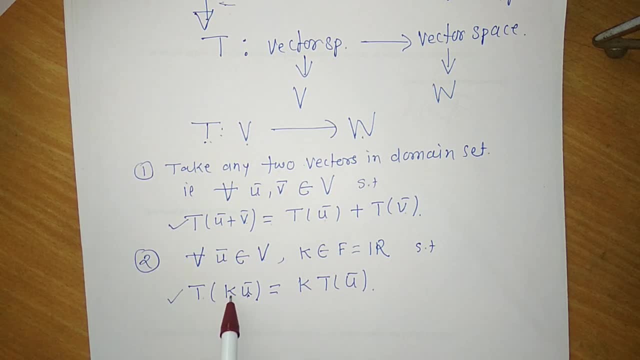 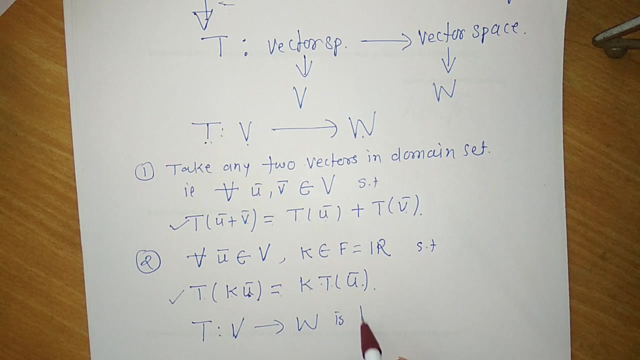 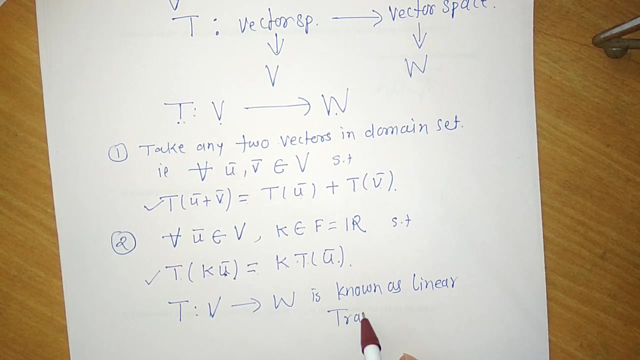 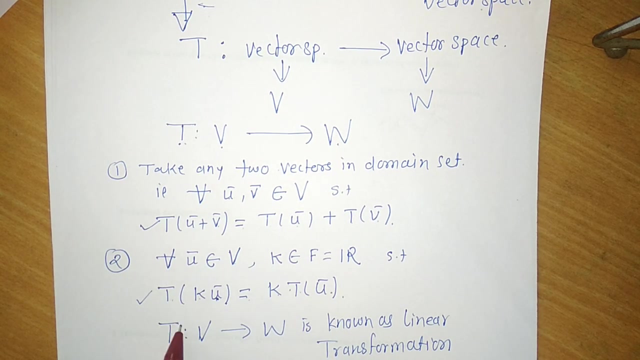 and second condition is that t of k times u bar equal to k times t of u bar. If any function satisfies the two, then such a function- t from one vector space, v to w- is known as linear transformation. If one of the condition is not satisfied, then such a function is not a. 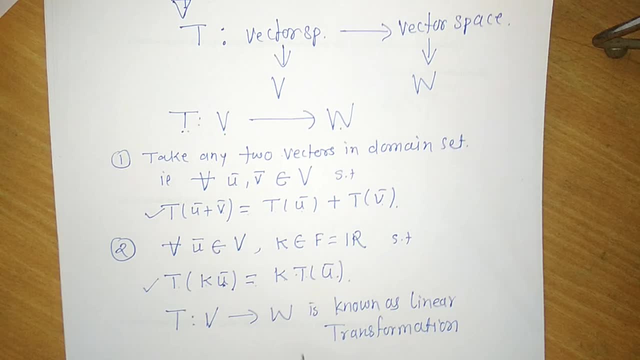 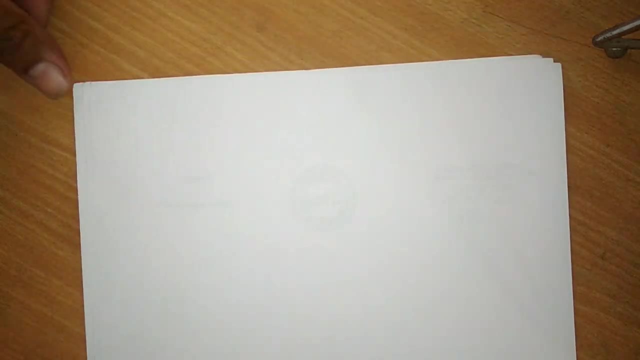 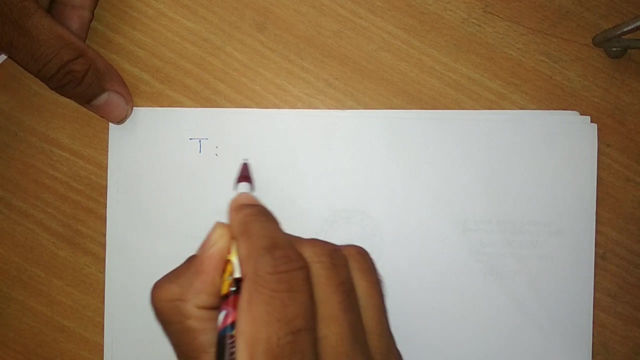 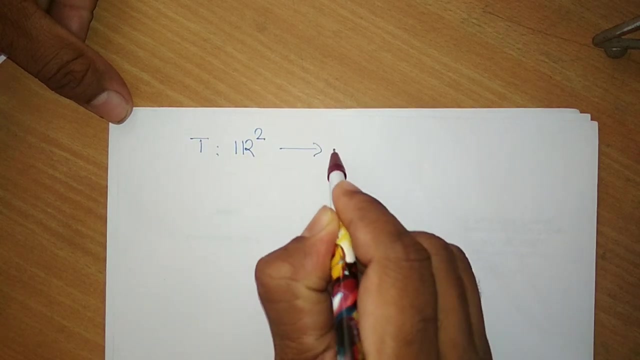 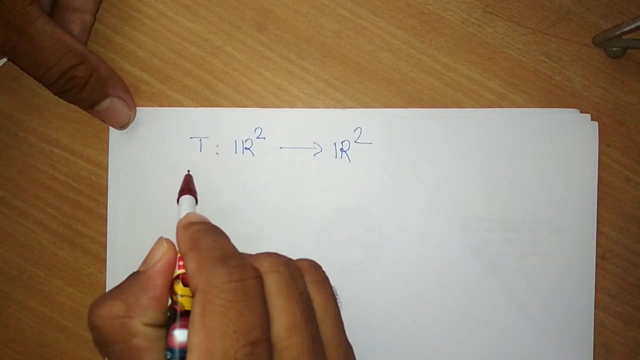 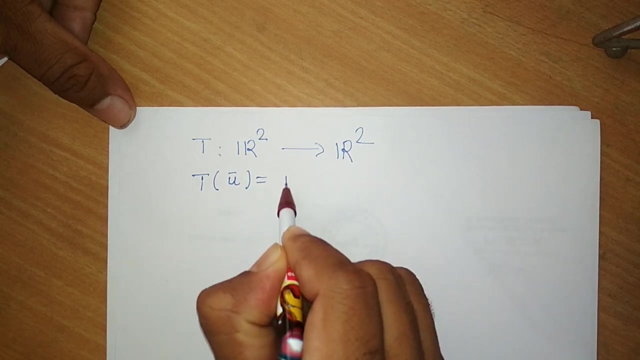 linear transformation. Okay, let us we consider the example. okay, suppose t is a function from one vector space, so domain is a vector space. so we consider the simple vector space R2, so domain is a vector space and codomain is also vector space. two dimensional: define the function: t of u bar is equal to, so t of u bar is a vector in R. raise to 2. 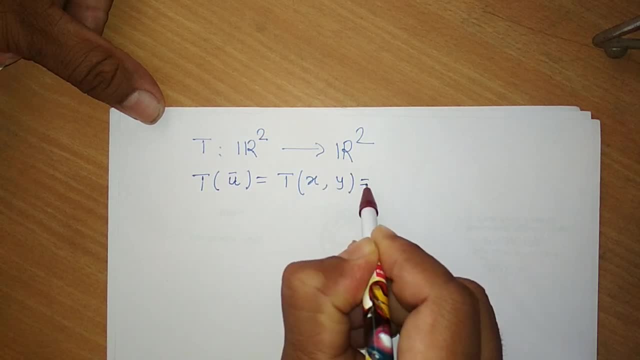 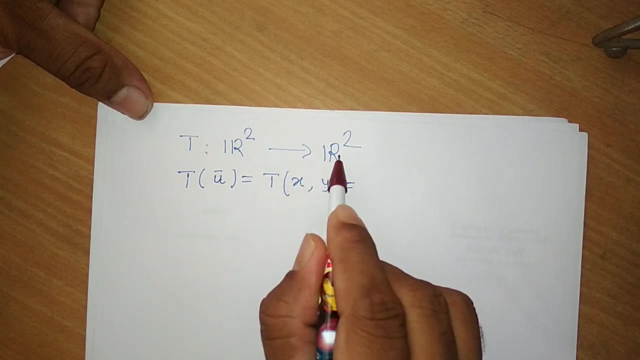 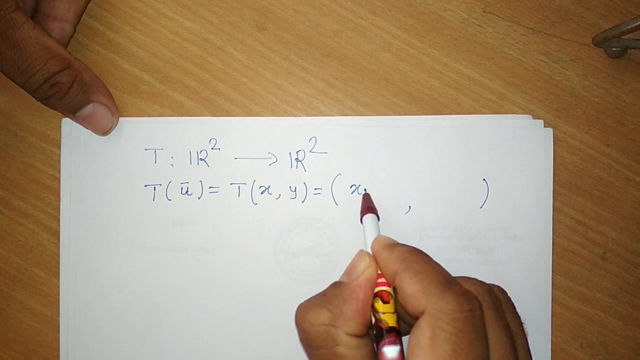 so u bar has two components, say x, comma, y equal to, so x, y is the vector in R2, so its image t of x, y is also a vector in R, raise to 2. so it has two components. so let us consider: the first component is x plus 2 y. 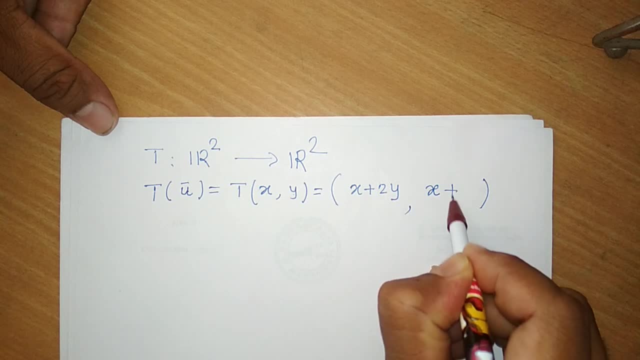 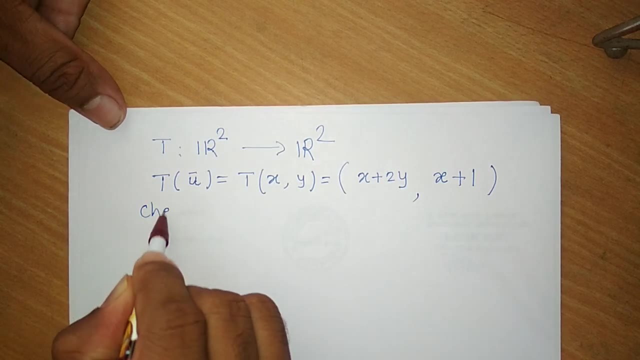 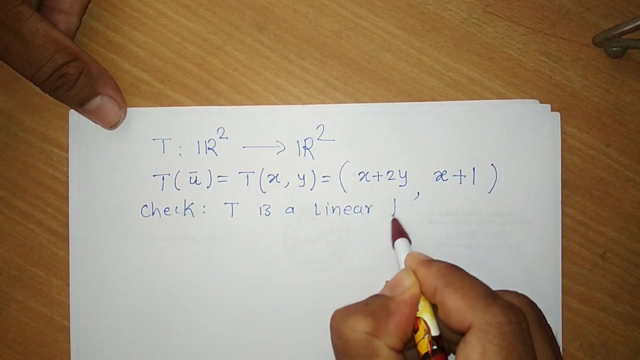 and here we consider x plus 1, consider this function in this way, and here we have to check, here to check, t is a linear transformation. okay, so it is clear that t is a function from one vector space to the another- in comingger to several cl익t of t, If any. 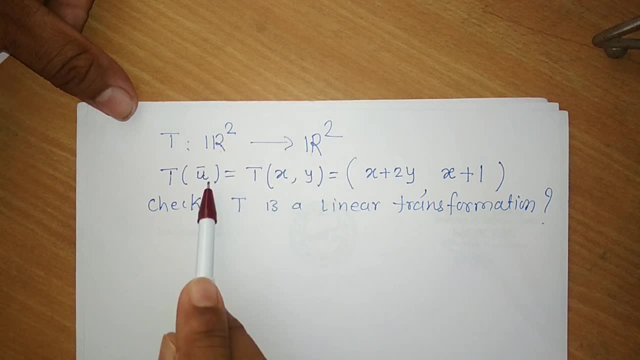 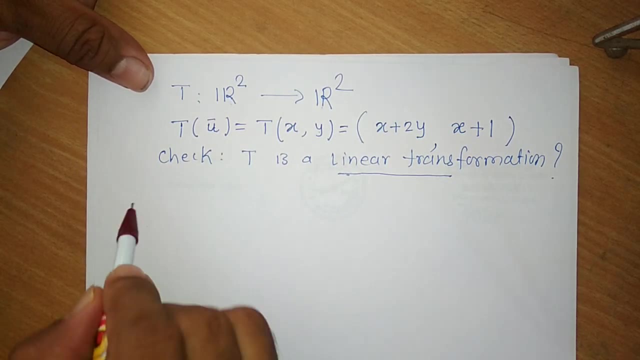 t is a function from two different vector spaces. so It is clear that t is a function from one vector- danger vector space defined by this function. we have to just take that such a function is a linear transformation or not. so we have to check the conditions we want to. 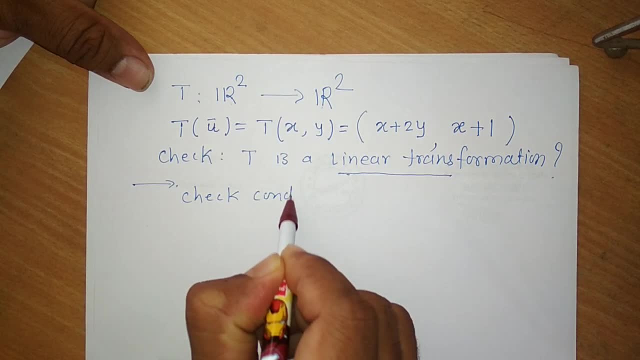 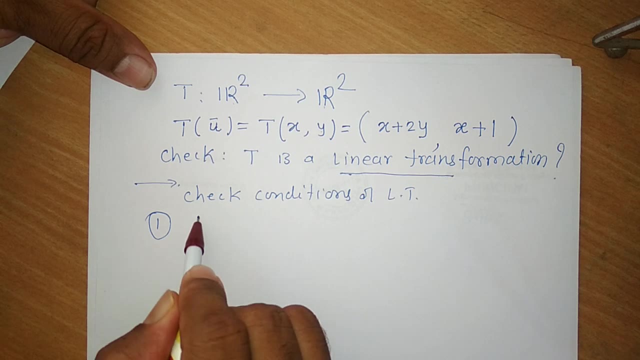 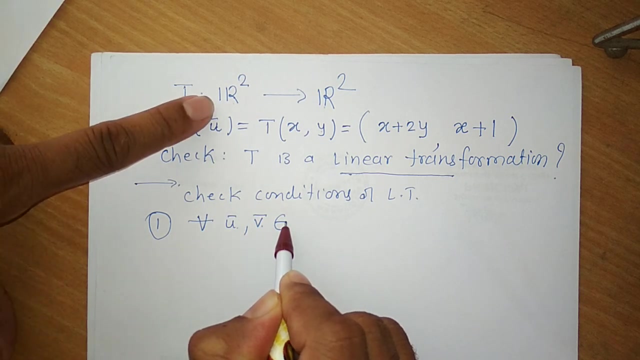 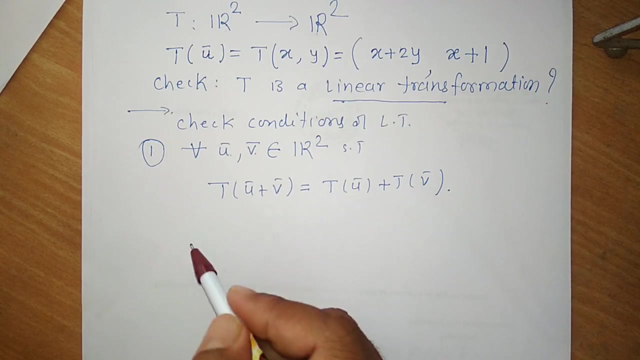 check the conditions. check conditions of linear transformation. the first condition is that take any two vector, u bar and V bar, in the domain set, that is, domain set is r raise to 2, such that T of u bar plus v bar must be equal to separate images, T of u bar plus T of v bar. okay, so let us consider: 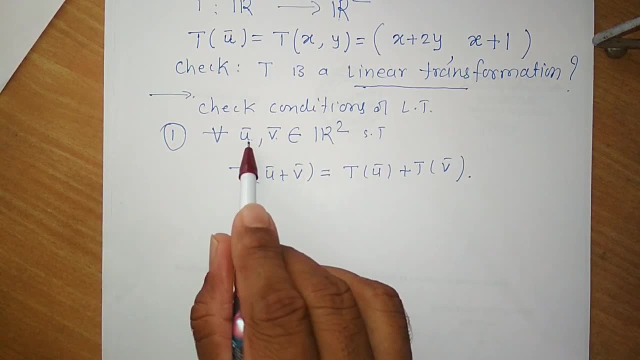 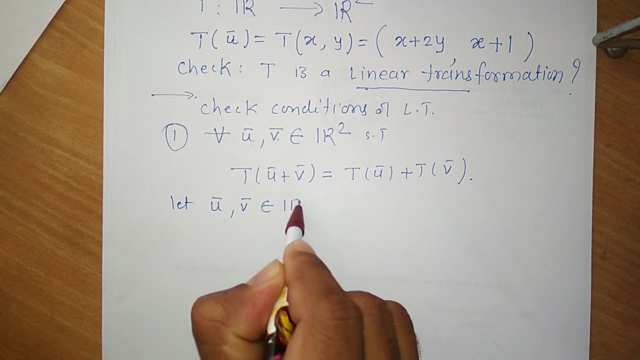 the two vector in are: should how to check this condition? so take the two vector in r raised to 2, let u bar and v bar are the two vector in r raised to 2, so u bar and v bar have a two components. see u bar equal to u1, u2 and v bar equal to v1, v2. these are the two vectors. 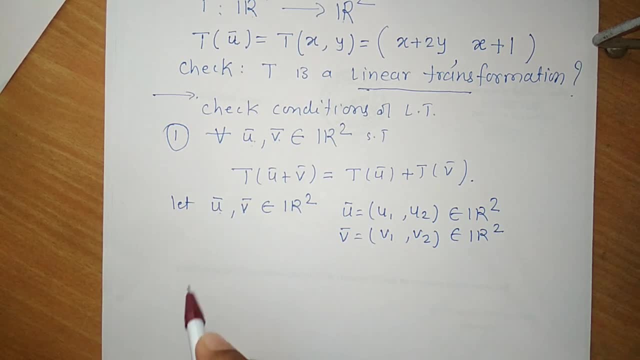 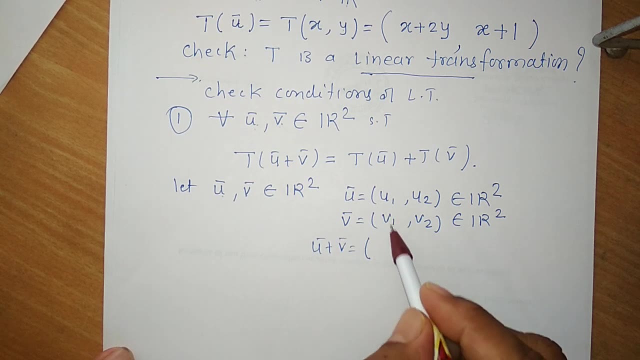 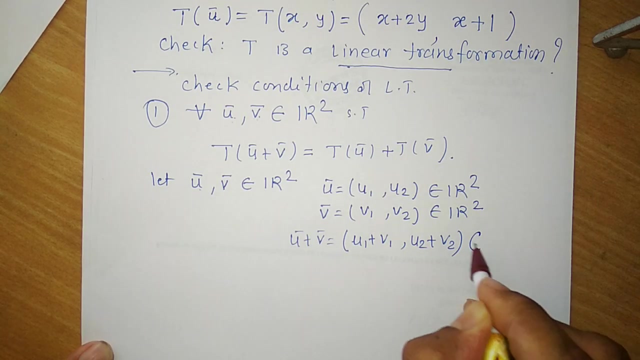 in the domain set, that is, r raise to 2. okay, we need to find u bar plus v bar, so u bar plus v bar equal to. we take the component wise addition: u1 plus v1 comma, u2 plus v2. this is also vector in. 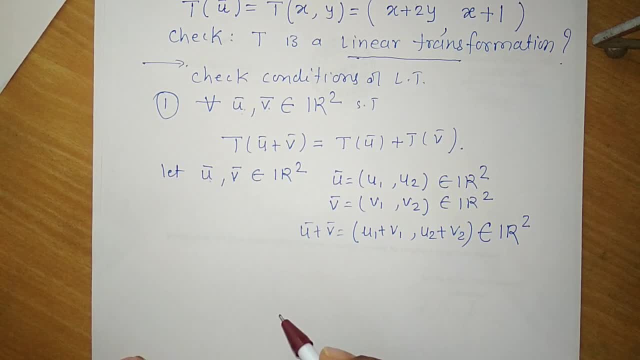 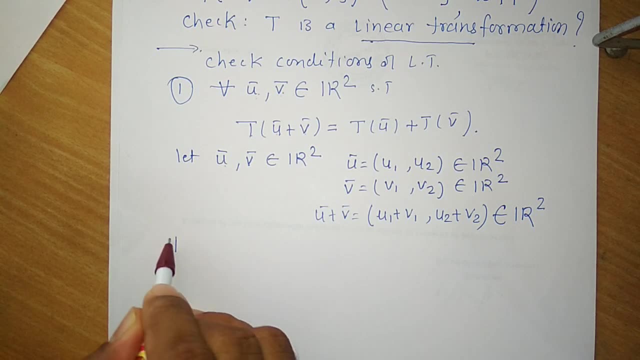 r raise to 2 because r raise to 2 is a vector space. now find out the image left side: t of u bar plus v bar. so t of u bar plus v bar, equal to t of u bar plus v bar, is already. this vector is: 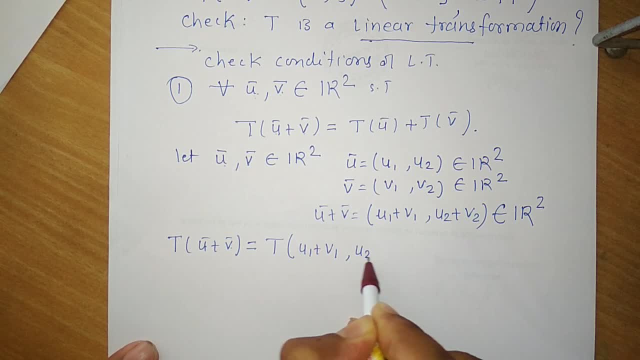 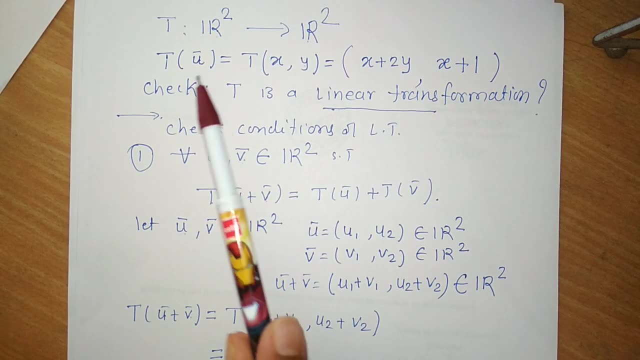 here. so u1 plus v1 and u2 plus v2, which is equal to. now see what is the function is given. so t of xy is equal to image of this vector is the first component is x plus 2y, the x plus 2 times. 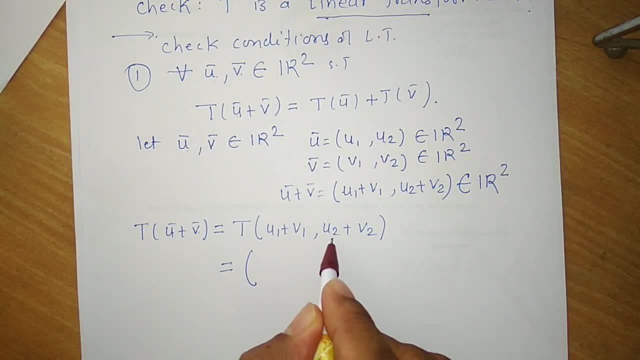 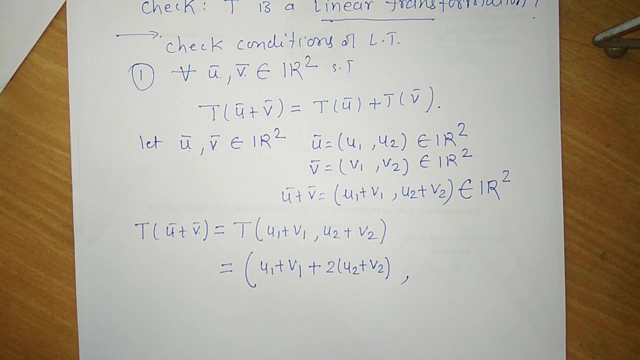 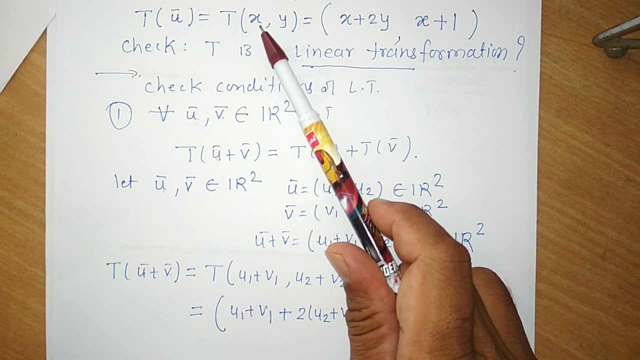 y. so here image of this vector is x plus 2 times y and the first u1 plus v1 plus 2 times this, 2 times u2 plus v2. this is the first component. and second component is if you observe that x plus 1, x plus 1 means the first component, the vector x added with 1. so here also the first. 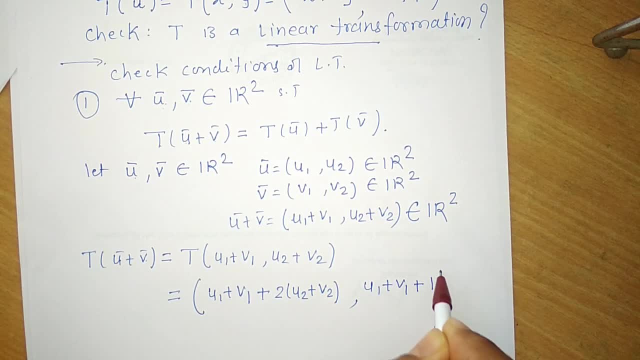 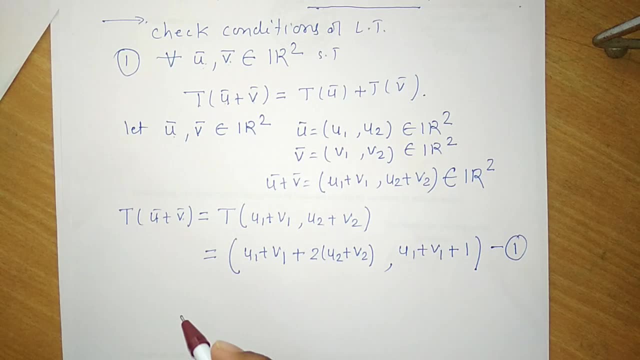 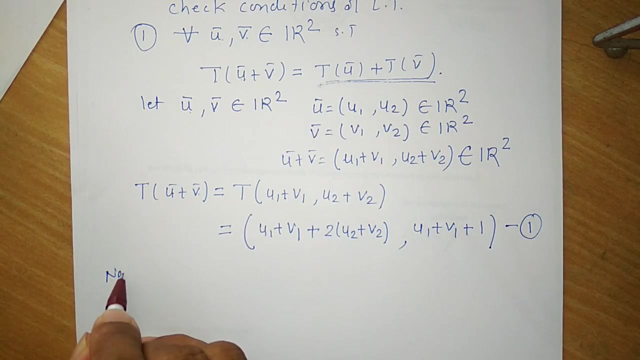 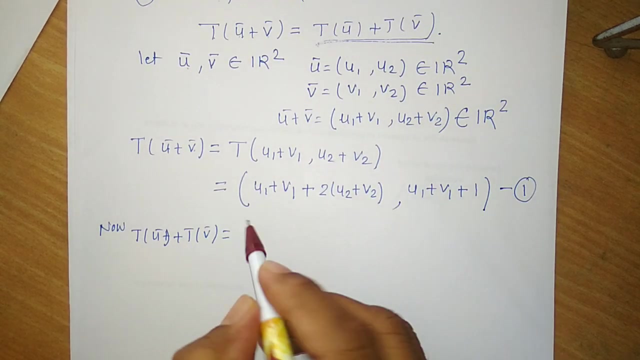 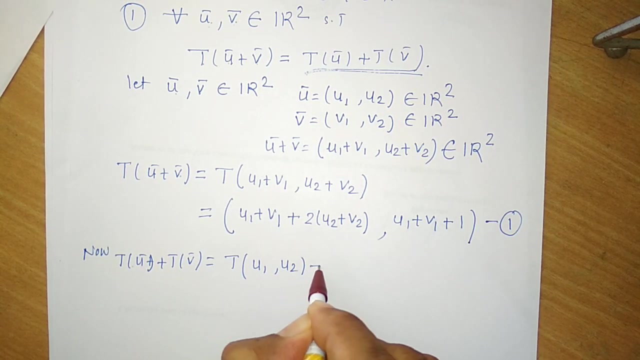 component is this: u1 plus v1 added with 1. okay, so this one is here. we call as a first equation: now we calculate the this side t of, now we can calculate the right side of that. t of u bar plus t of v bar equal to t of u bar means u1, u2, u1, u2 plus t of v bar means: 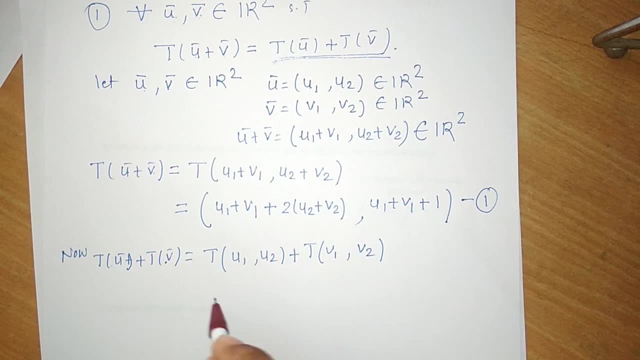 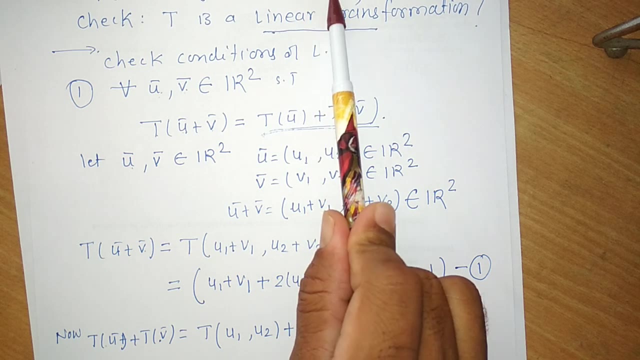 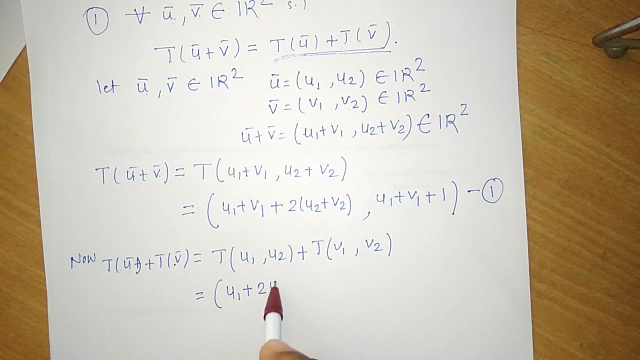 v1, v2, v1, v2. now we find out the images of this and the function is given: t of xy is x plus 2y. so this is x means u1 plus 2y, 2 times y means u2. second component: x plus 1. the vector whose. 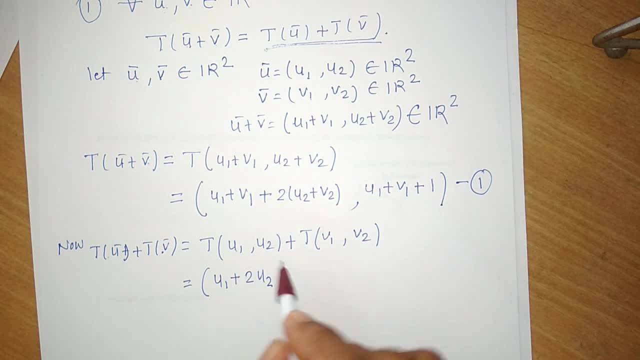 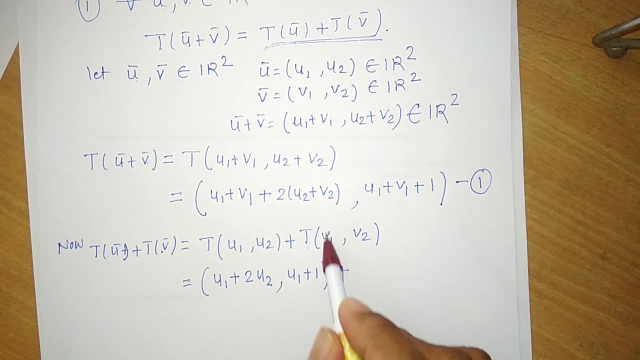 first component, x plus, added with 1. so your first component is u1 plus 1 plus. similarly, we can calculate the image of this vector: v1, v2. under t, the formula is given that x plus 2y. x means v1 plus 2 times. 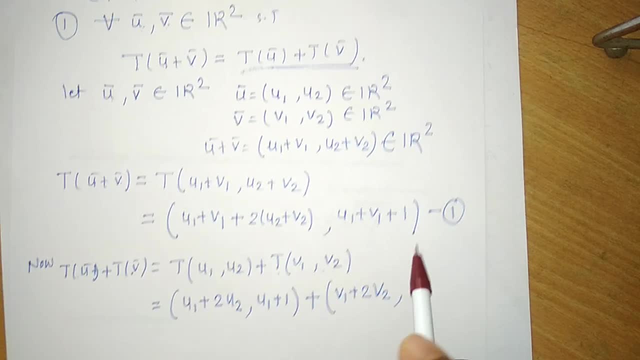 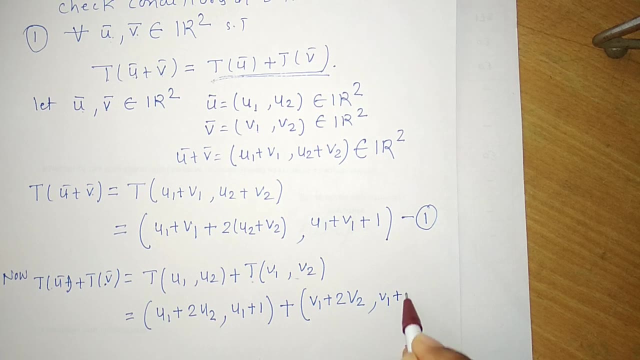 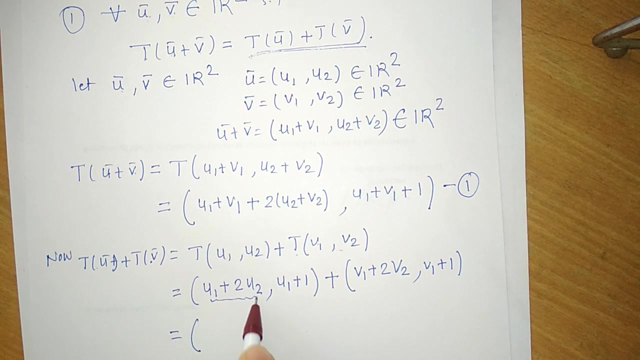 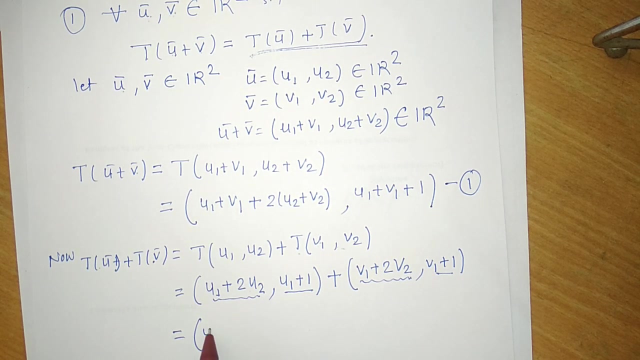 v2 and the second component is here: x plus 1. the x component added with 1, x component, v1 added with 1. now we add these two vectors here. component y: this component is added to this component. this component is added to this. so u1 plus 2 times u2. 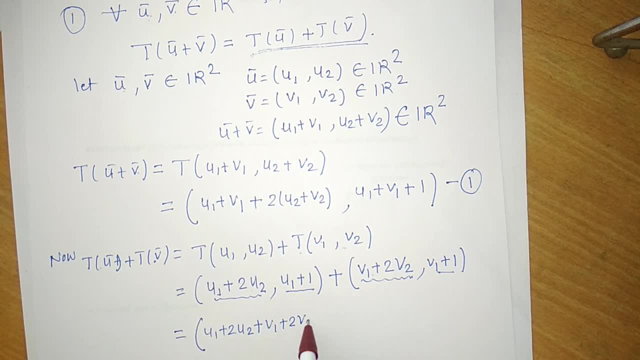 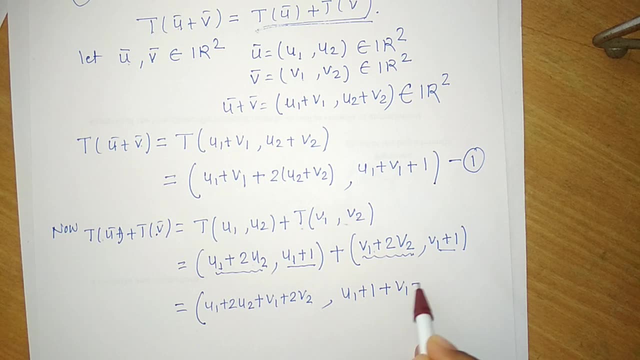 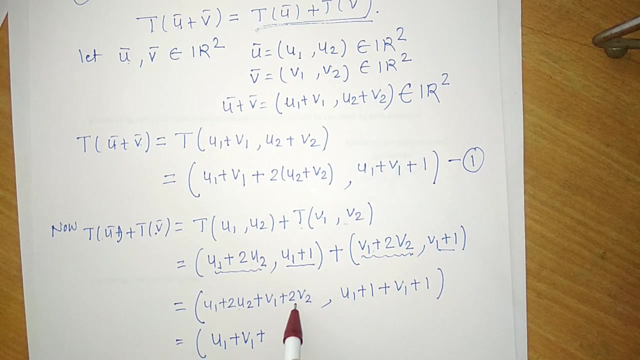 plus v1 plus 2 times v2. second, u1 plus 1 plus v1 plus 1. if we simplify what happened: u1 plus v1 plus, you can take the 2 is common: u2 plus v2. u1 plus v1 plus 1 plus 1 is 2, we call as a 2, now we 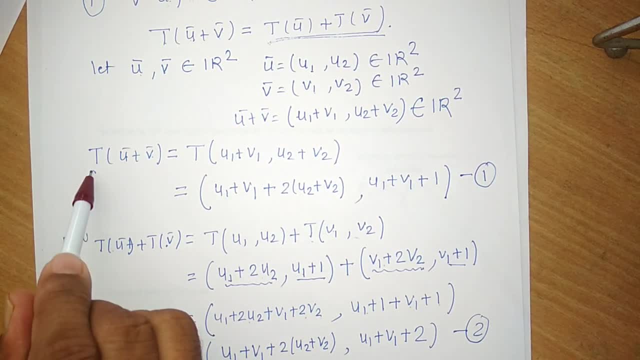 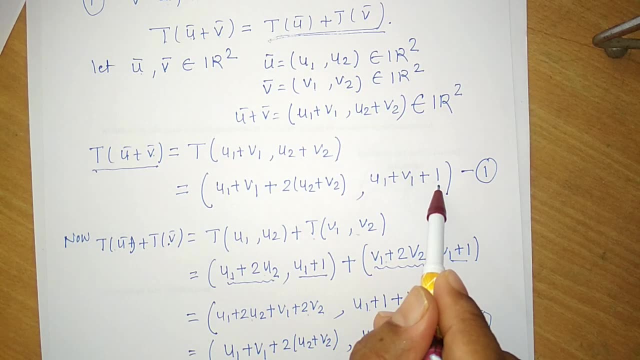 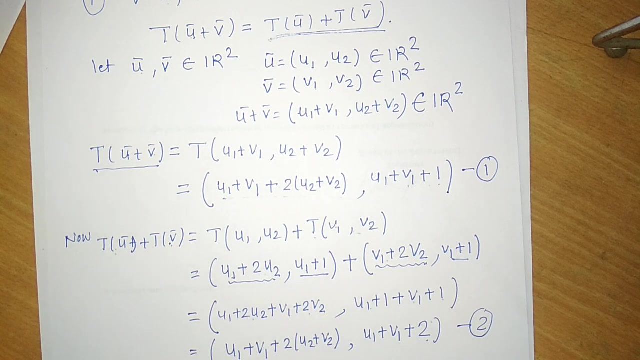 observe here. so this is t of u bar plus v bar and its image. is this vector? okay, and t of u bar plus t of v bar. we calculate this image: is this vector? if you observe these two vector equation, one and two, the first components are same: u1 plus v1, two times this u1 plus v1. 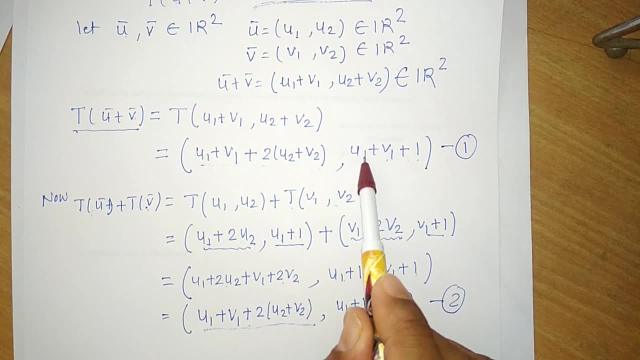 two times this. but the second component: here u1 plus v1 plus 1 and here u1 plus v1 plus 2, so this is 1 and this is 2. the second component of these are not equal, so these two vectors are not equal. 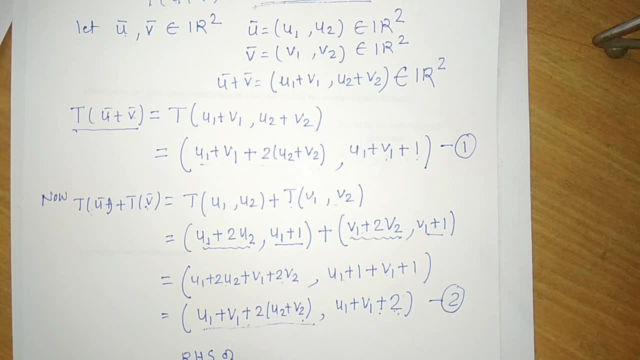 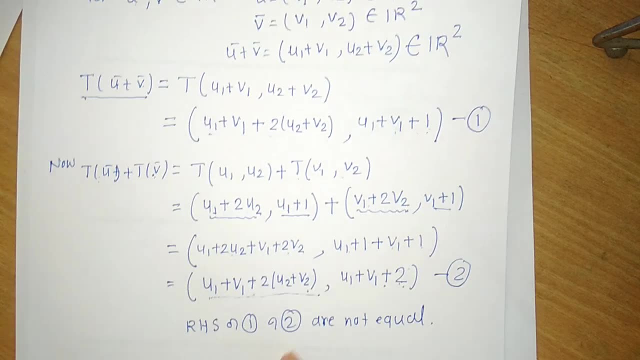 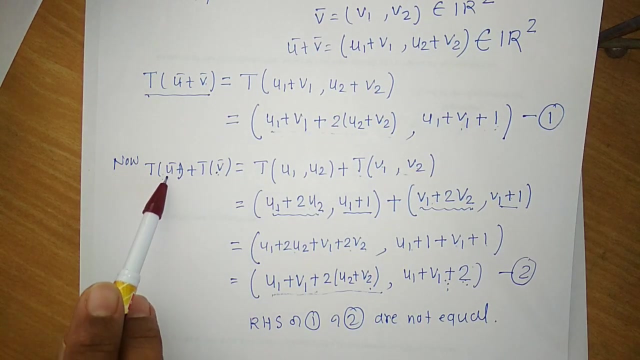 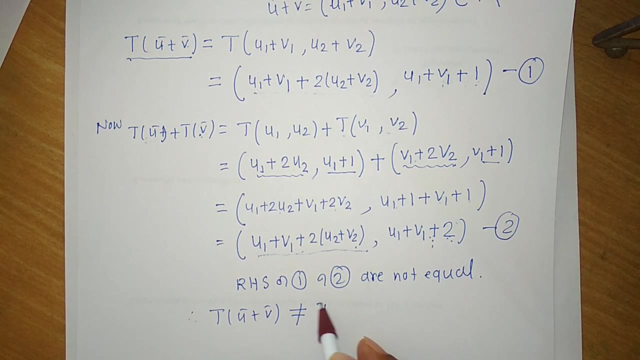 so right hand side of 1 and 2 are not equal, not equal. therefore their left side, these two equations, their left side means t of u bar plus v bar and u plus tv. therefore, t of u bar plus v bar is not equal to t of u bar plus t of v bar. therefore, 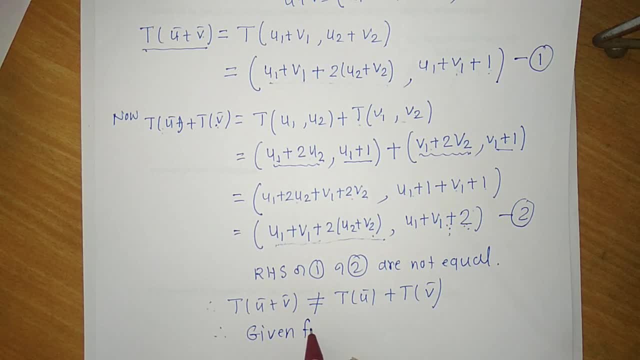 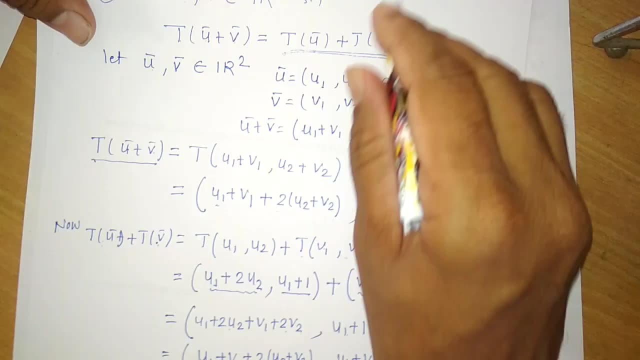 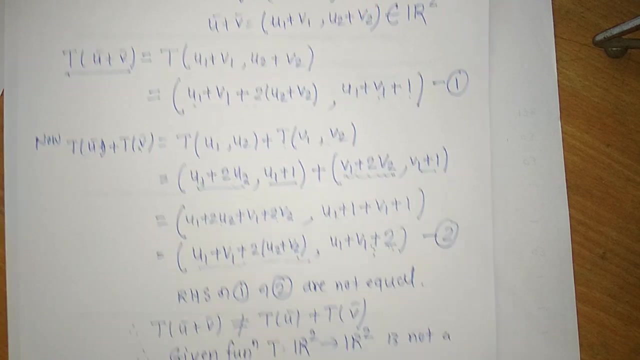 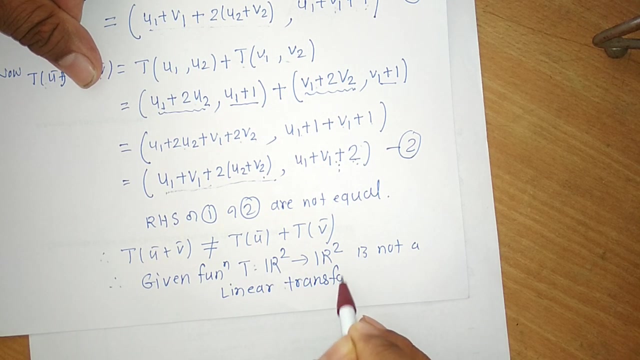 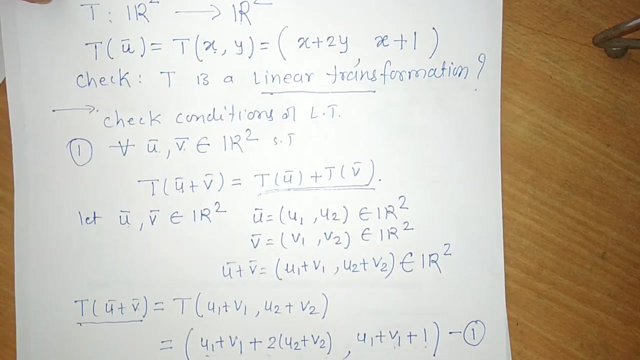 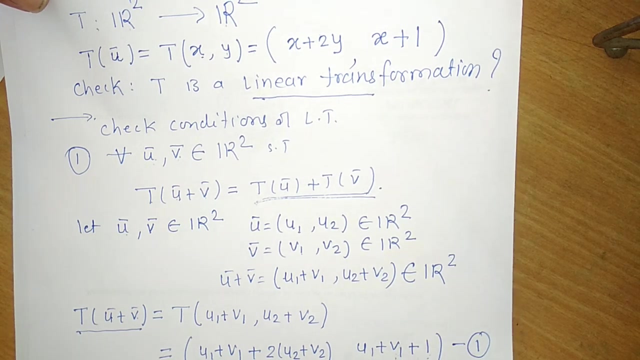 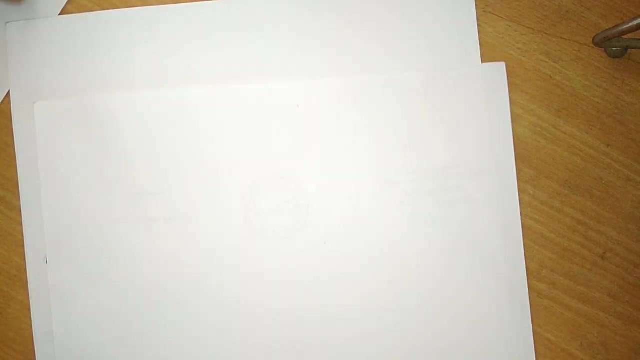 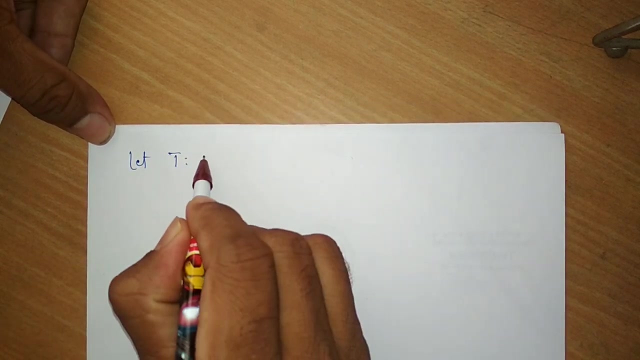 the given function, given function t from vector space r2 to r2 defined in this way, okay, is not. a is not a linear transformation. so this is very good example that this function is not a linear transformation. now let us consider the another example. let t is a function from one vector space, r2, to the another vector space, r2. 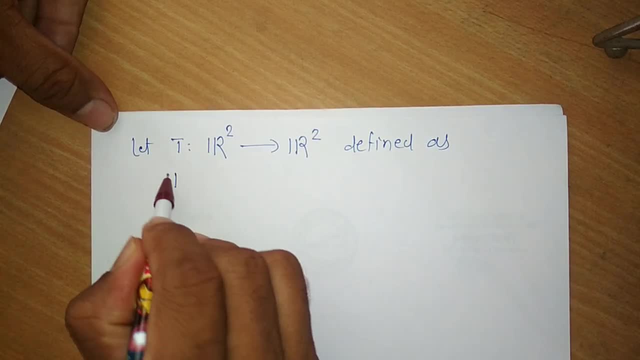 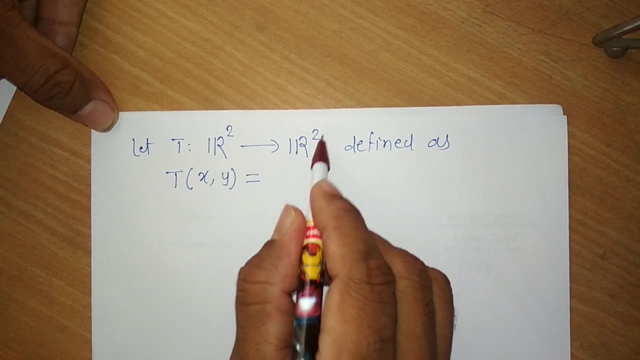 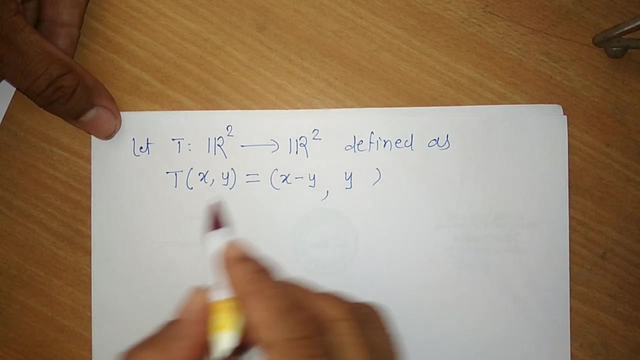 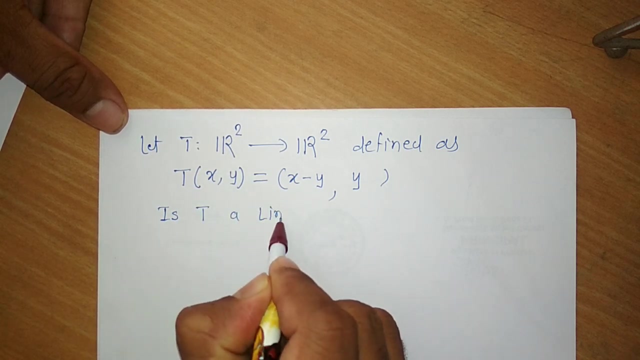 defined as this function, defined as t of. so take any vector in r2. its components say x, y is equal to its image. is the vector in r2, it has a two component. so we consider x minus y and here we consider y. the problem is that is such a function, is t a linear transformation? 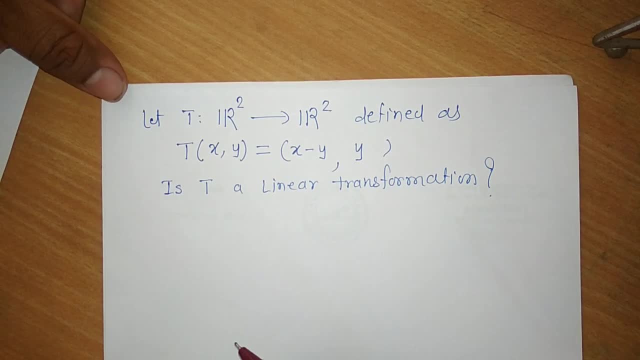 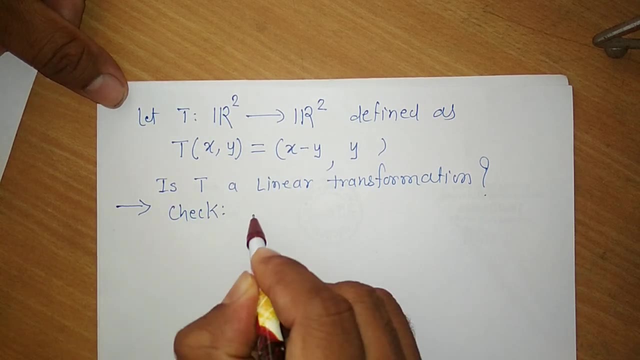 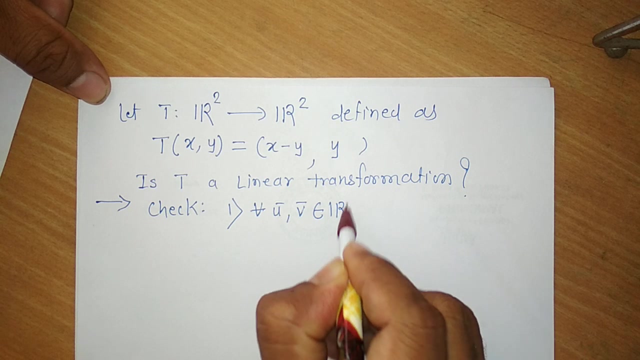 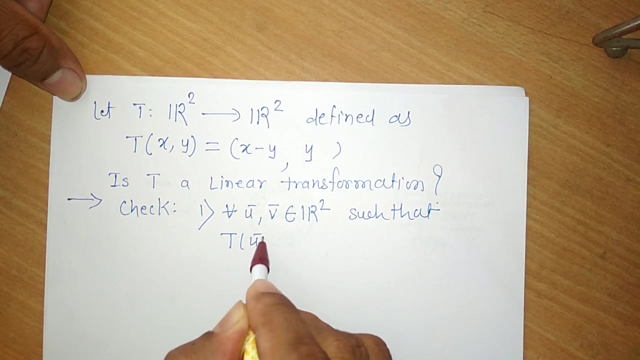 linear transformation question mark. so again we have to check the conditions. yeah, two conditions. what you have to check. first condition is: take any two vector- u bar and v bar is in the domain r, raised to two, such that t of u bar plus v bar is equal to separate images. 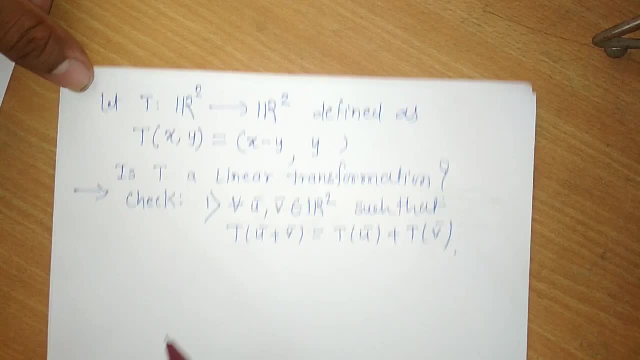 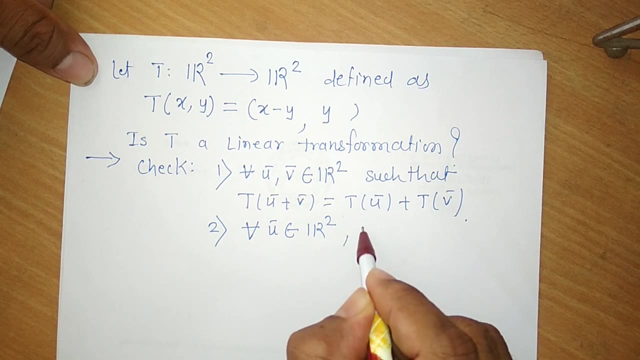 t of u bar plus t times v bar. and the second condition is that take any vector u bar in the domain set. r is to take any scalar k belongs to field a, and suppose the field is a real number such that t of k u bar is time k times t of u bar. so we have to check the two conditions here. 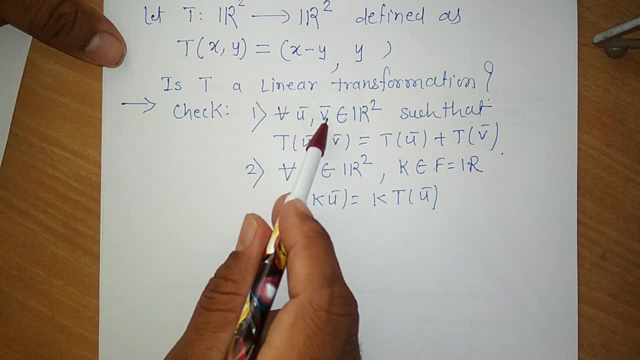 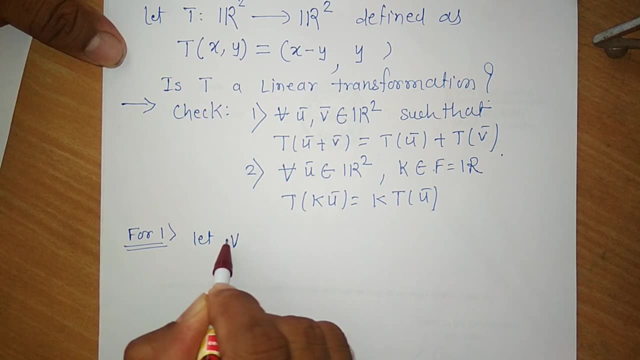 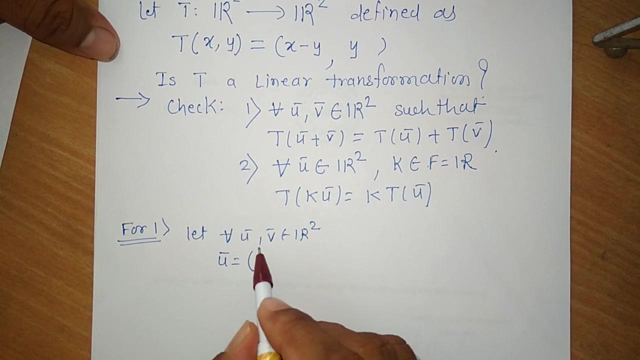 so we check the first condition for that. we need the two vector in rs2. for first condition let any two vector, u bar and v bar, in rs2, as u bar is the vector i also i consider here a x1, y1. suppose the vector v bar is x2, y2. these are the two vector in rs2. that is the domain set. 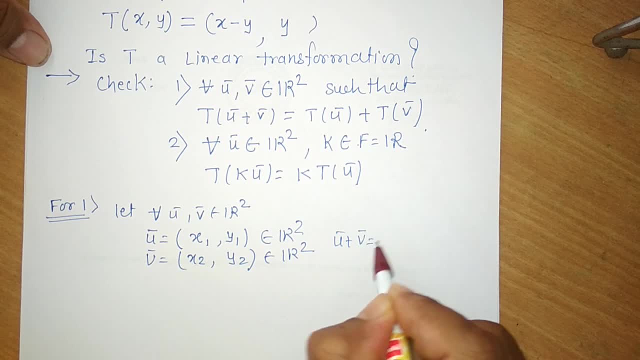 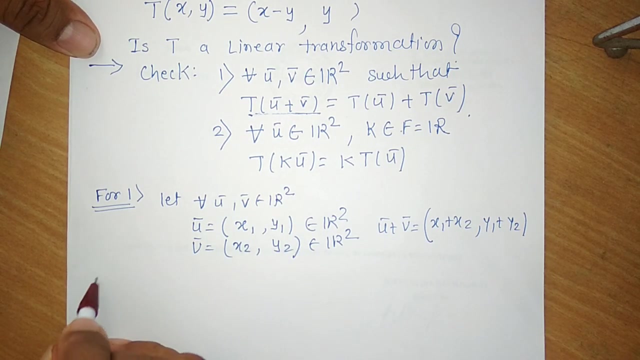 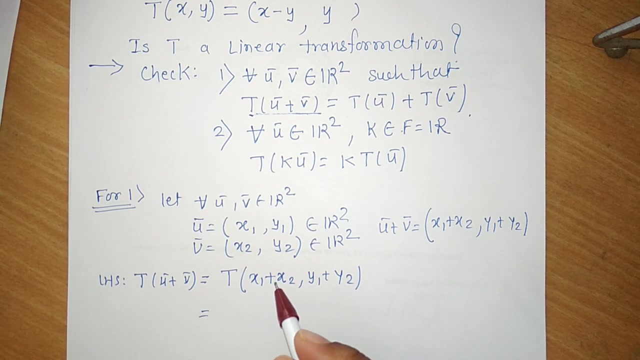 we find out their addition: u bar plus u bar, because that addition is we required here: x1 plus x2, component y and comma y1 plus y2. now we find out the Golfлас zia after y isso. we eliminate them all. yeah, now we had removed the the. 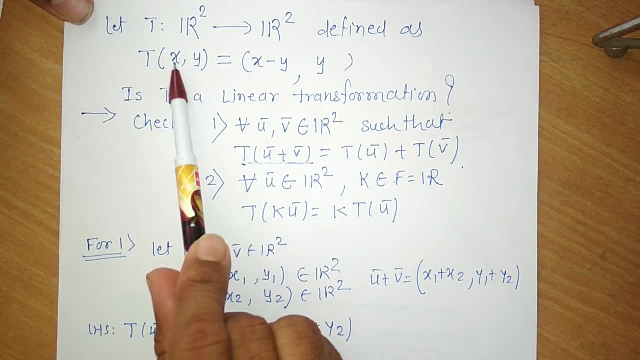 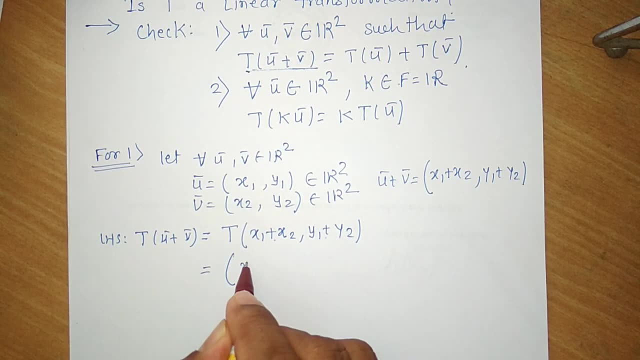 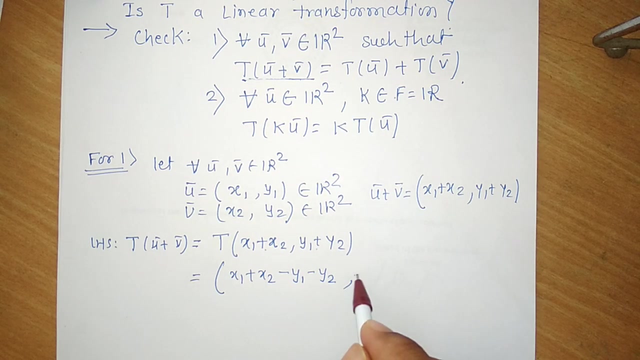 is first component is X minus. I'm just subtraction of these two component comma. second component, as it is the same here, the subtraction of these X 1 plus X 2, subtraction minus Y 1 minus Y 2 comma. and second component is as it is and we 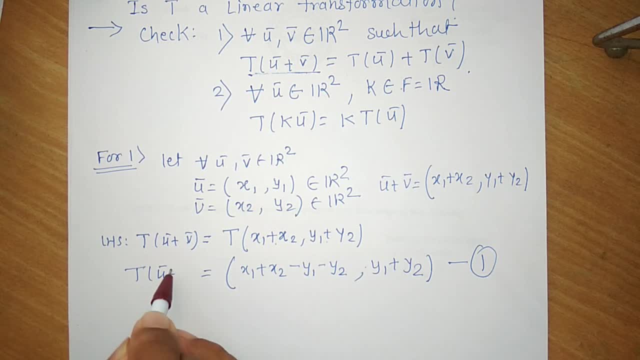 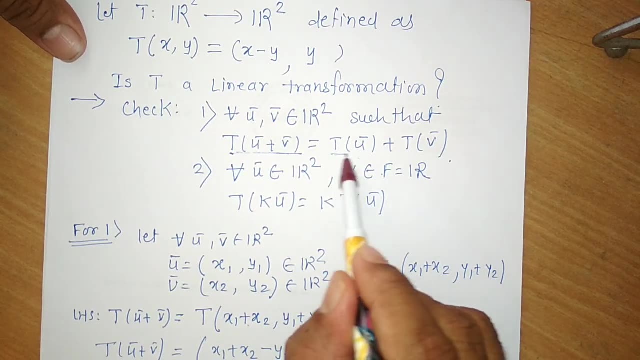 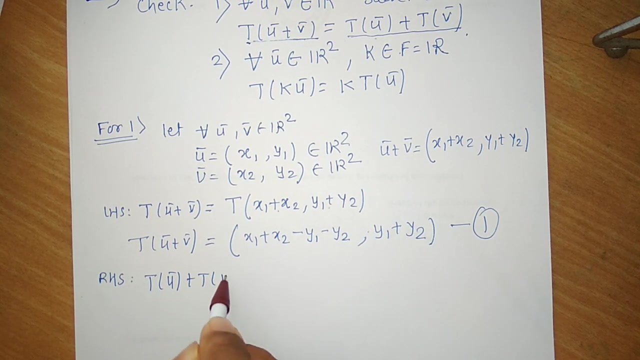 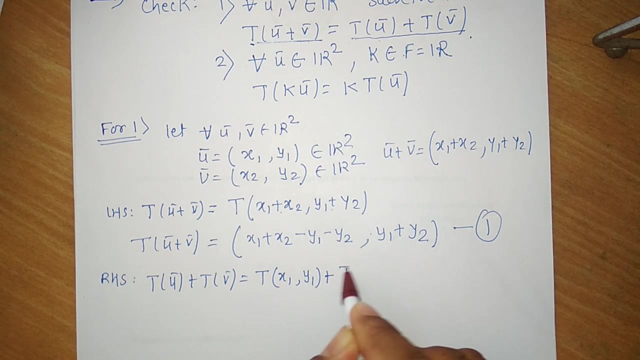 call that the first here. now we evaluate the right side of that right side, side of this side, T of u bar and c of u bar. T of u bar means X Y 1 plus T of u bar. vector means X 2 Y 2. we. 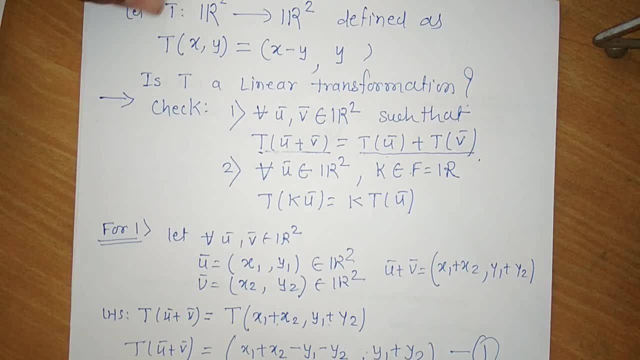 evaluate the image of this vector under T formula is here T of XY, means the first component is subtraction X minus Y comma into the first bracket. Now here wethe other side ofática is from the equation X plus X minus Y, And in the previous example we saw, though, if we solve the terms not equal to 2 times. 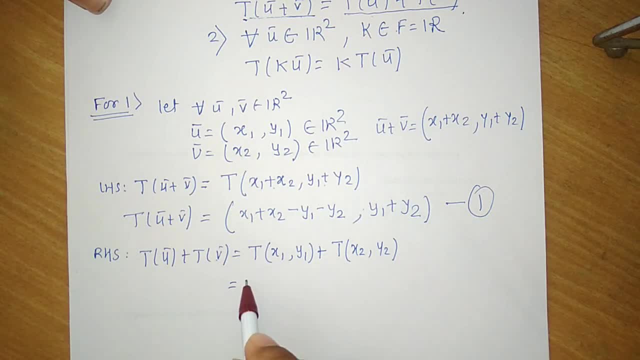 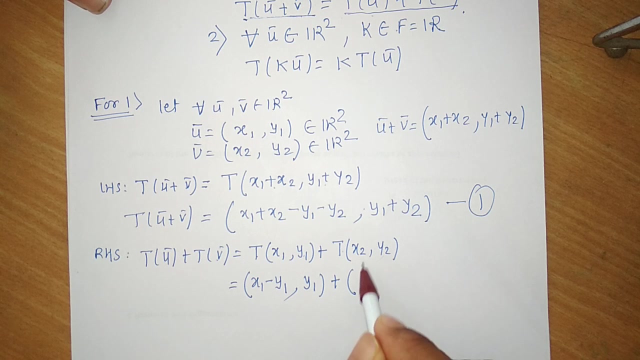 a y component as it is. in the same way, t of this vector is x1 minus y1 and second component is y1 as it is plus t of this vector. that is the image of this vector under t formula is defined above that subtraction of the two x2 minus y2 and second component, y2. 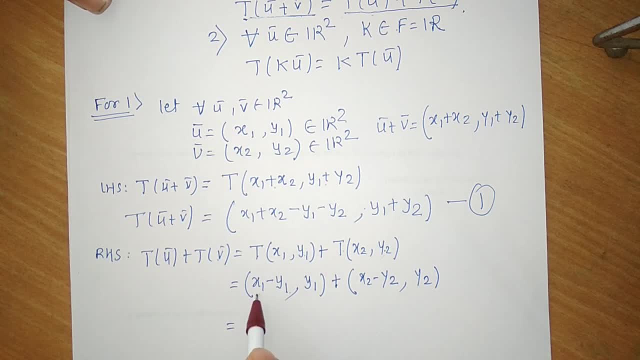 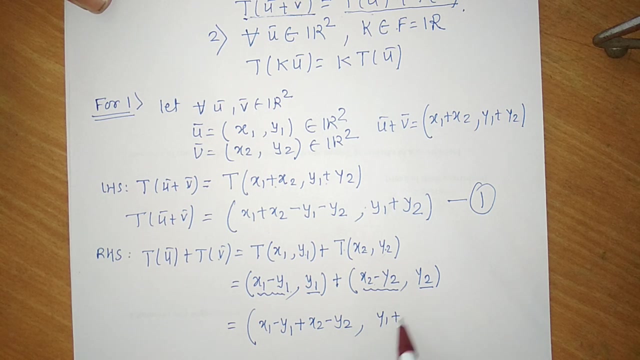 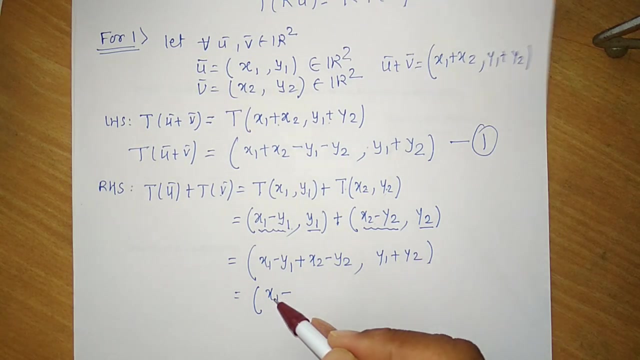 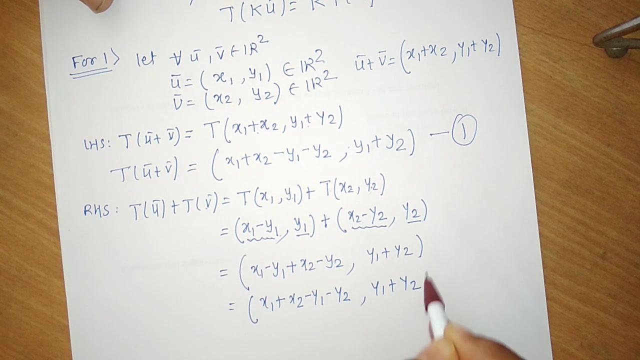 we add the two vectors. so addition is component wise. add the first component and add the this. so x1 minus y1 plus x2 minus y2, y1 plus y2. so we simplify: x1 plus x2 here minus y1 minus y2, y1 plus y2. so we call as a two. and if you observe the one and two, the right side. 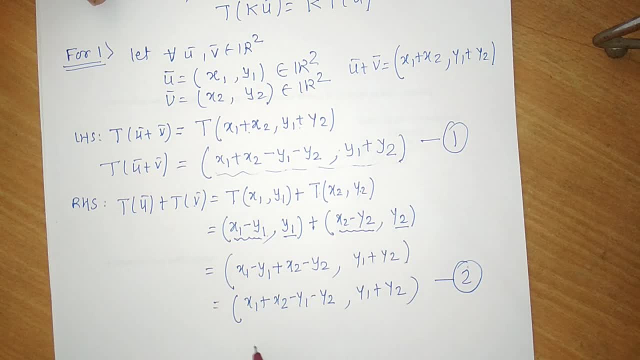 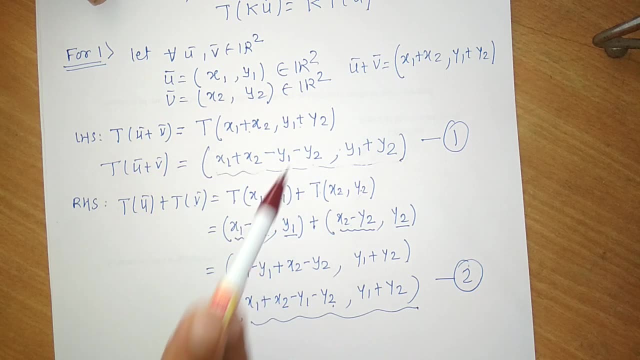 this vector has a two component and this vector has also two component, both vector, whose first component is x1 plus x2 minus y1 minus y2. here x1 plus x2 minus y1 minus y2, the second component is also same. therefore these two vectors are same. and if the two vectors are same, then their left side. 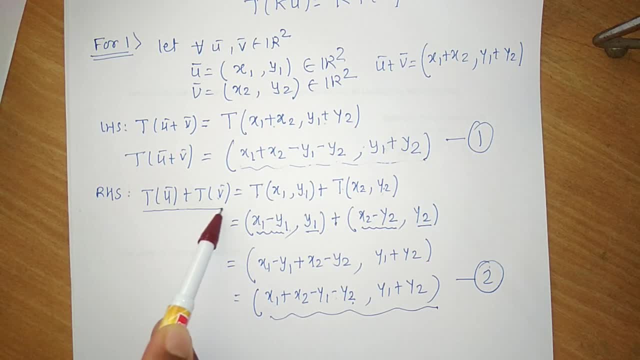 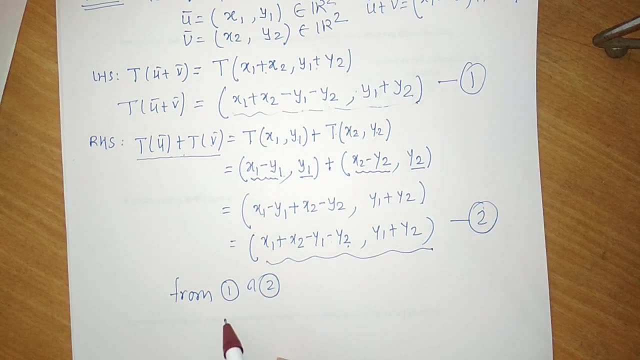 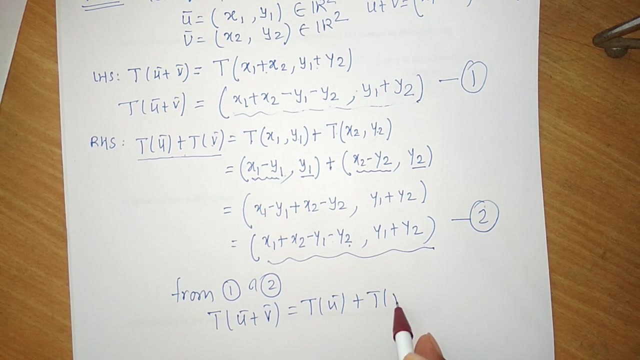 t of u bar plus v bar and t of u bar plus t of v bar. they are same. therefore, from one and two we write. from one and two we write: t of u bar plus v bar is equal to separate images: t of u bar plus t of v bar. so in this way the first condition is satisfied here. 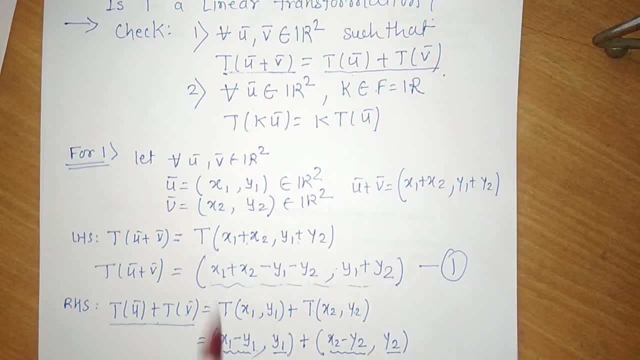 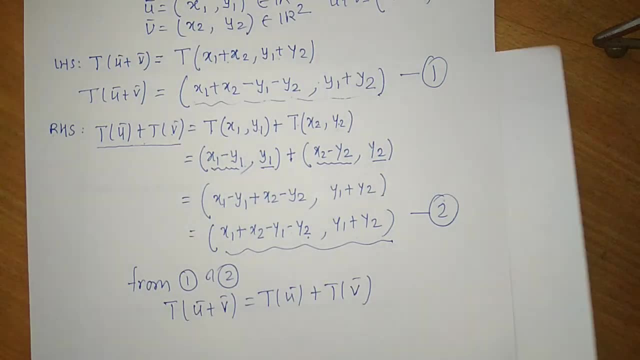 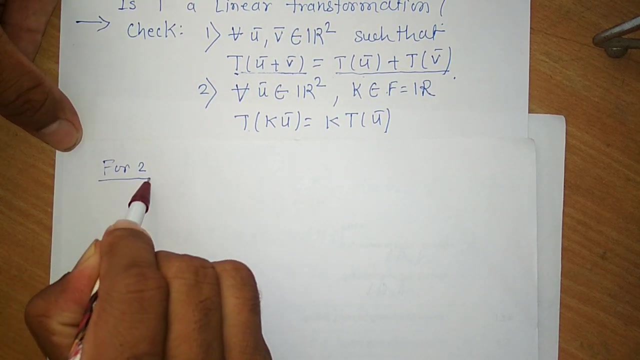 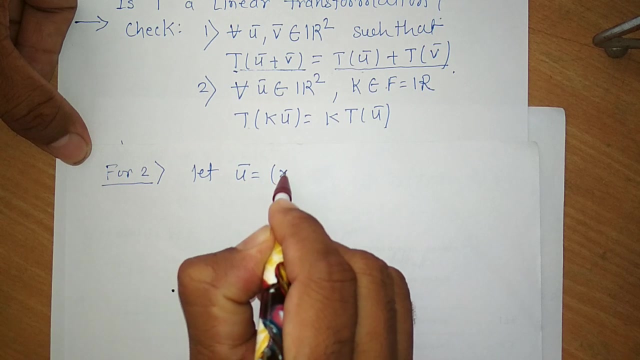 now we check the second condition. second condition is t of k? u bar is k times t of u bar. so for second condition, okay, so we need a one vector. u bar is r, let u bar is the vector. it has a component, say x1, y1 belongs to r, r2, that is the domain set. 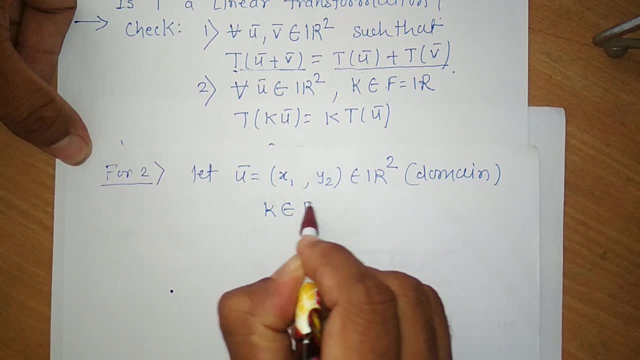 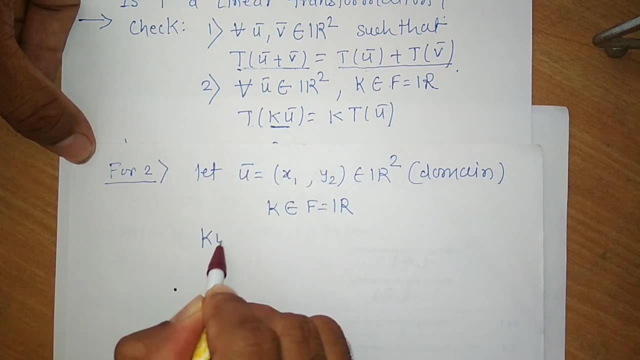 this is a domain set. we need a one scalar. say k belongs to f and field is real number. let us consider k times u bar. we need this. k? u bar is k times u bar means k? u bar. vector means x1, comma, y1 and the scalar multiplication of the vector. so, as usual, that k is multiplied to the. 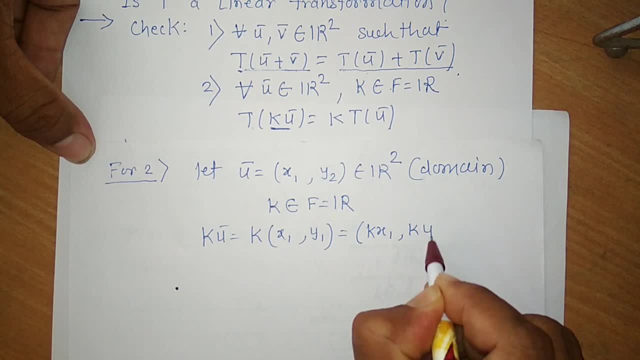 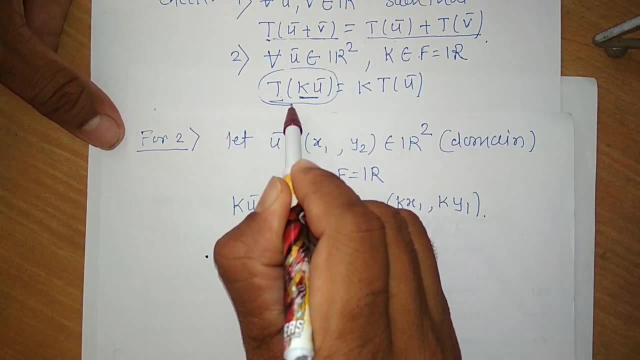 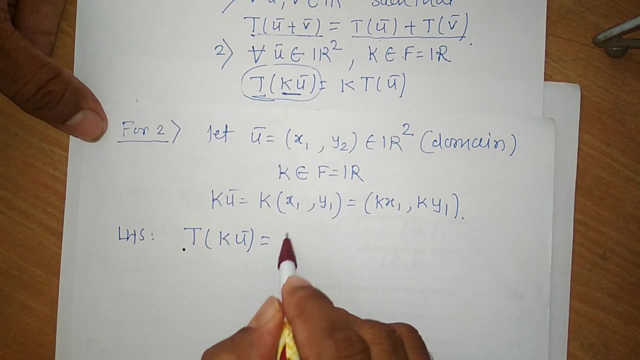 every component of that vector, that is k, x1, k, y1. okay, now we consider the left side of this: t times k u bar: x1 normal is equal to the left side. t times k u bar equal to t of k? u bar means we already. 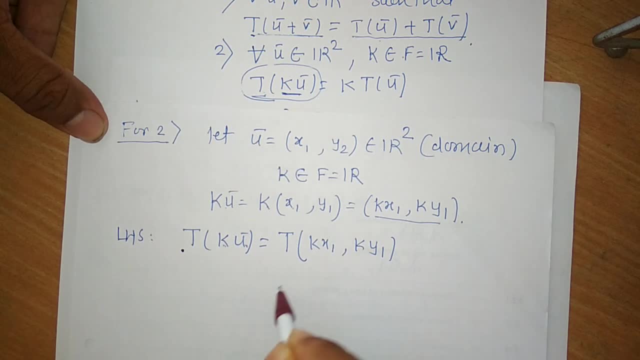 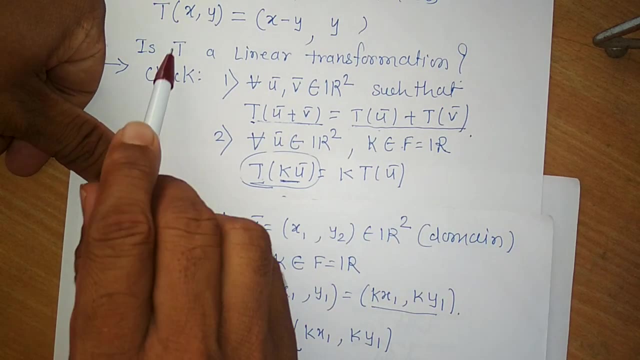 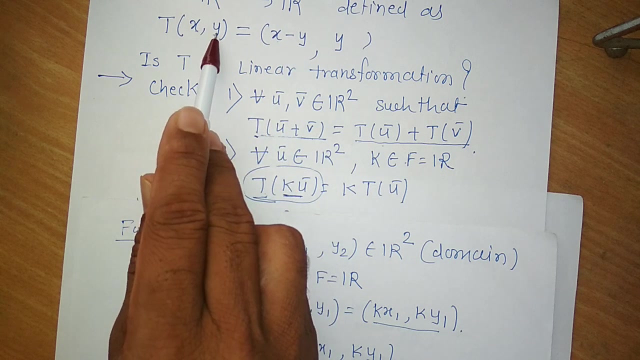 even this is the vectors you can write here: k, x1, k, y1. equal to what is the image of this vector under t? the formula is given here: t of xy is equal to x minus y, which is subtraction of the two comma y component. as it is. 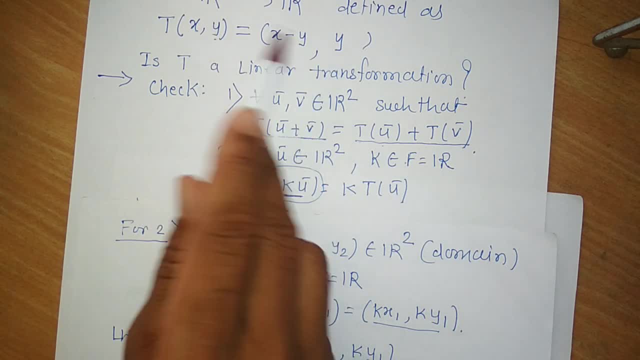 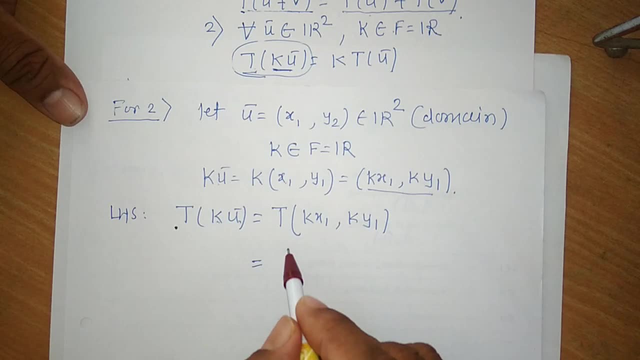 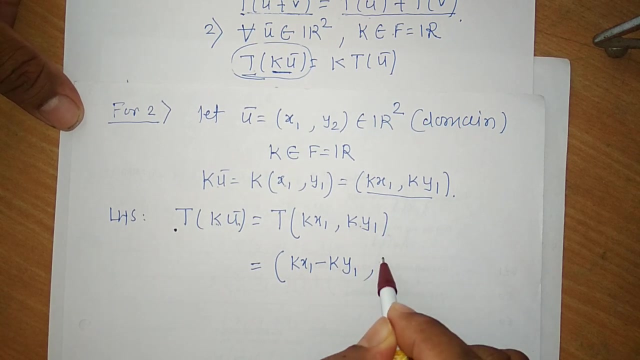 the this: In this example the function is defined in this way. okay, So we consider here subtraction of this kx1 minus ky1, and second component is ky1.. This vector is the image of this vector under D. So this is the vector in domain and this is vector in codomain set. 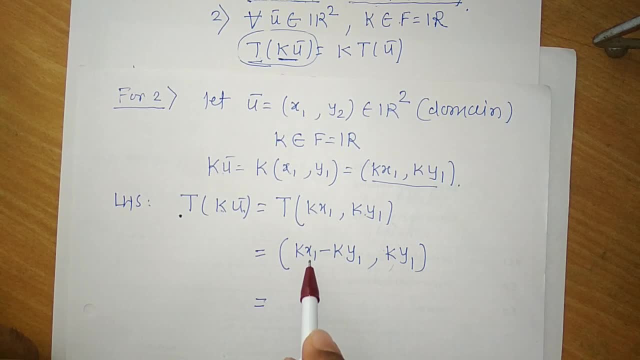 So if we observe that in the first component there are two terms and in the two terms k is the same multiplier factor, We can take the k is outside here from the first component. Similarly, if we observe that k is also multiplied to the second component, so we also take the k is outside. 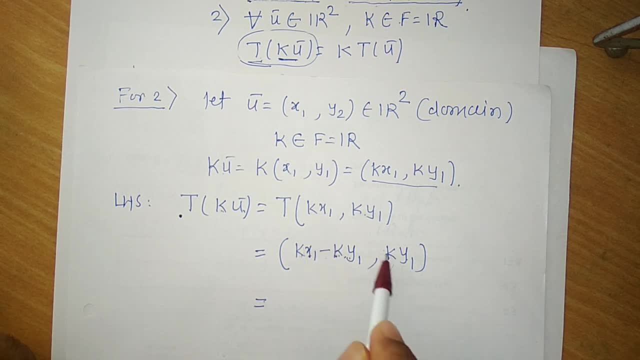 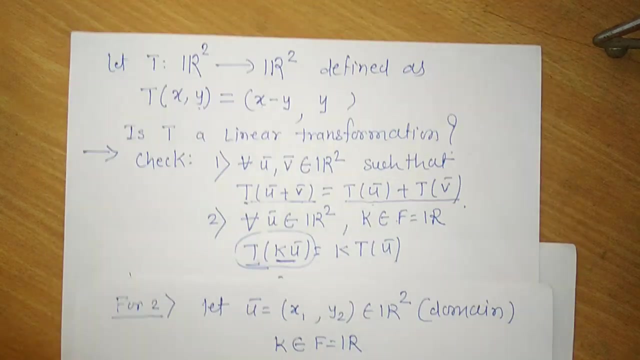 So in the first component k is outside, second is k. so take k is outside. second is outside here. so k times here: x1 minus y1 comma y1.. So k. so if you observe that this is the image of which vector, If you observe here x minus y comma, y is the vector which. 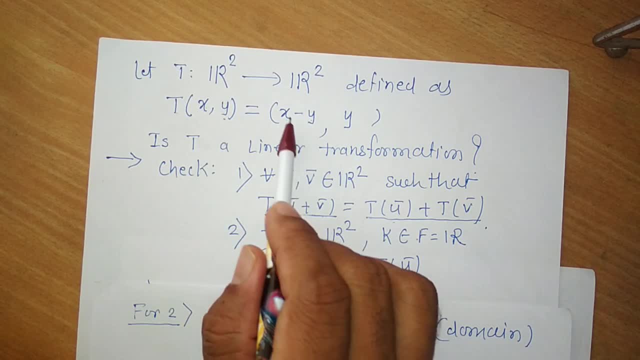 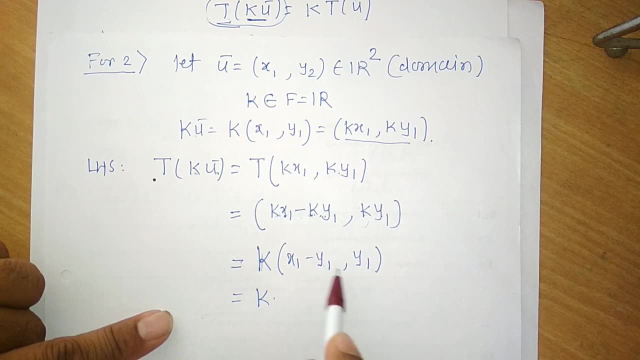 is the image of xy under t. So if it is a vector, then we write this vector as T of xy. in the same way, x1 minus y1 comma y1 is the vector 00,00,00 We can write: 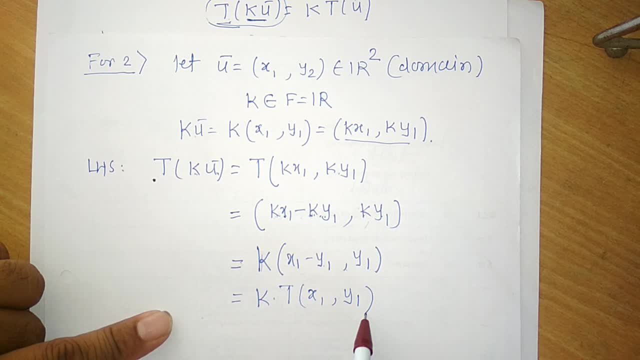 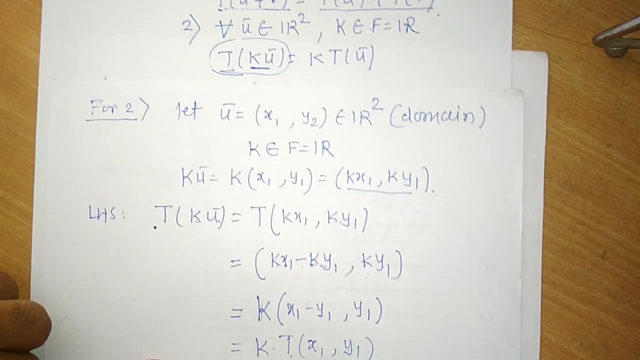 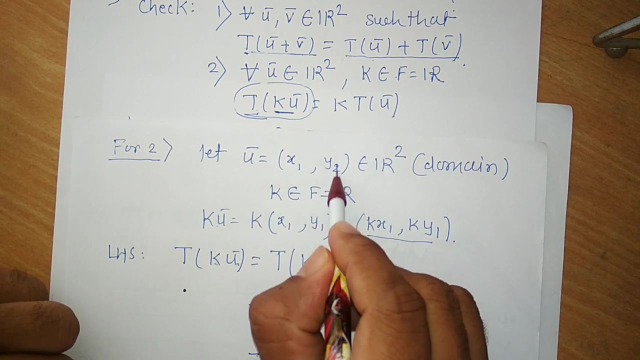 it as T of x1, y1. So this vector is the image of x1, y1 under T. So this is kT, and already we call x1, y1 means which vector u bar. So you will be like this: So T of u bar. So which is. 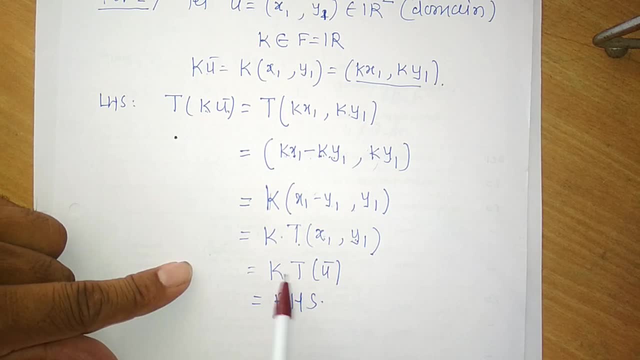 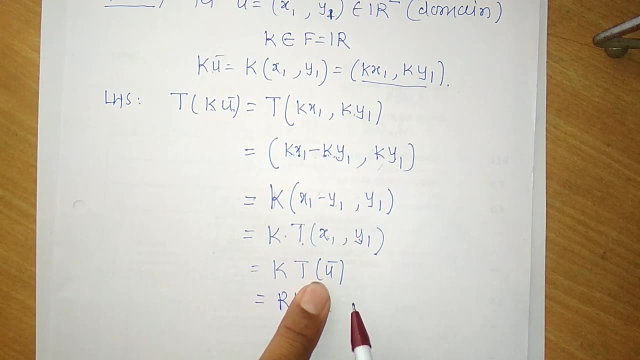 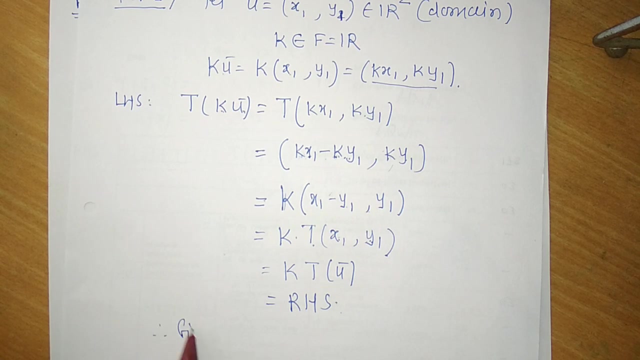 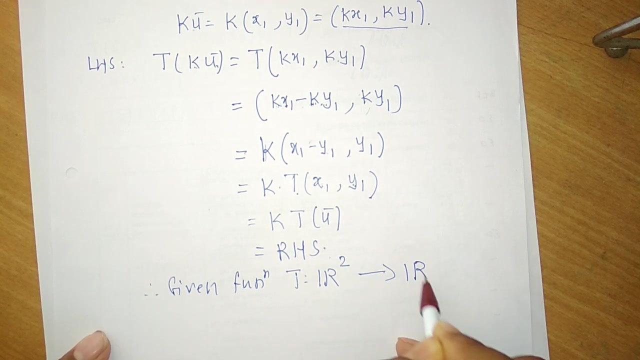 equal to right side of that which is equal to right side, k times T u bar, Hence T of k? u bar. after simplification, we get k times T u bar, Hence the function is also satisfied. The second condition, therefore: given function T from R2 to R2, that is, one vector space to another vector. 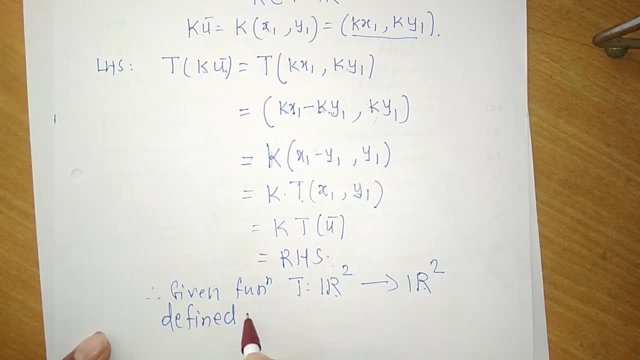 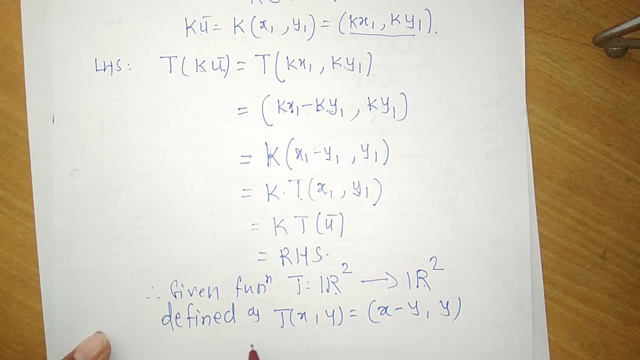 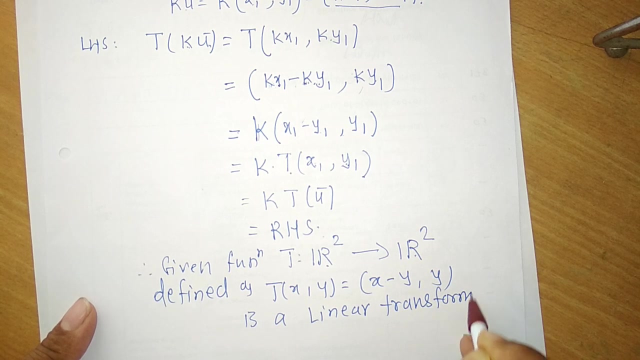 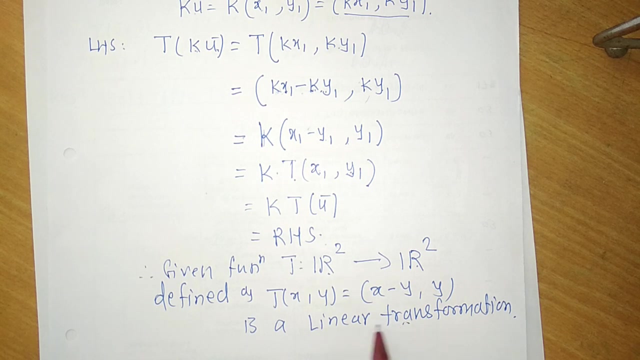 space define as T of xy is equal to x minus y. y is a linear transformation. It is a linear transformation. The linear transformation is always defined. it is always depends on how you define the function. So in this example, if we define in this way, then it satisfies all the two conditions. Therefore it is a linear. 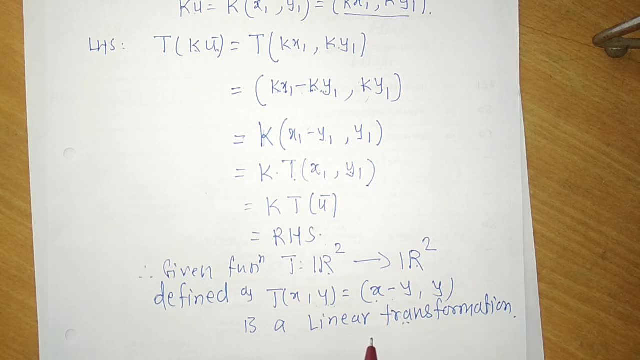 transformation. So today here we discuss what is a linear transformation and we also consider the two examples here. One is a vector space and another is not a vector space. Thank you very much. 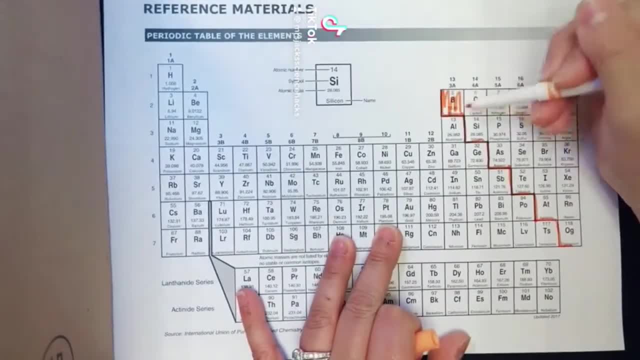 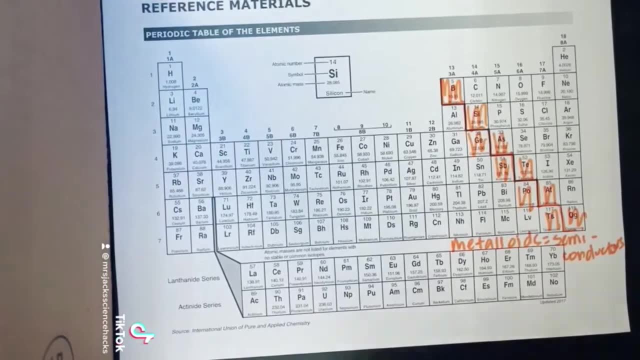 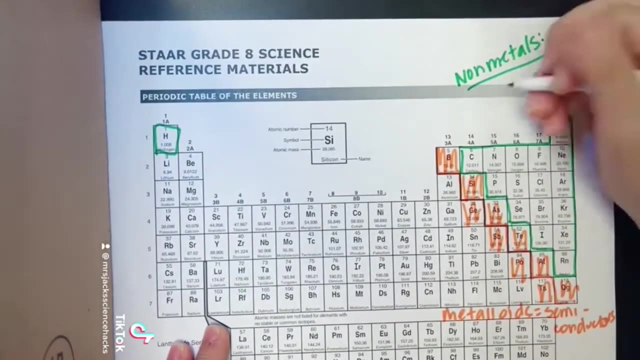 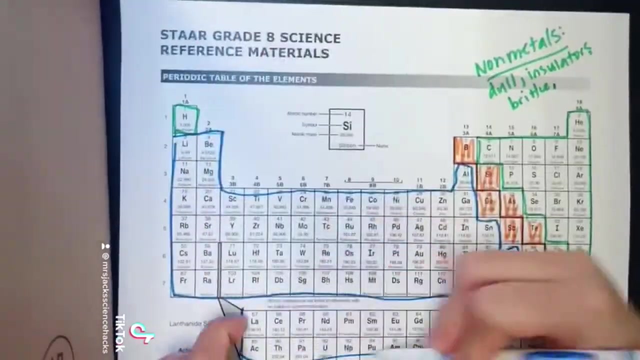 This is how you label the periodic table. First you start with the staircase. Everything on top and bottom of the staircase, except for aluminum, are metalloids. Their main property is they are semiconductors. Next, on the right side of the periodic table, we have our non-metals- Everything on that side plus hydrogen. their main characters are their dull, their insulators and they are brittle. Now the big chunk of the periodic table, most of these elements. they are going to be metals. Their main properties are luster, malleable and they are brittle.